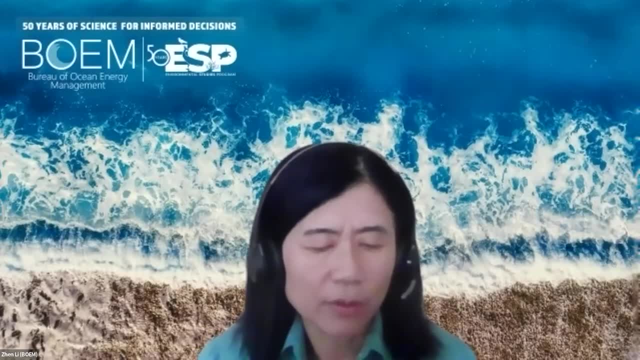 Physical oceanography team is now known as physical oceanography community of practice. Our team aims to coordinate research of the physical oceanography of the Arctic Ocean. Today, we'll be talking about the blue economy in Alaska. The ocean economy, also known as the blue economy, plays a pivotal part in Alaska's economy, as well as the entire nation. 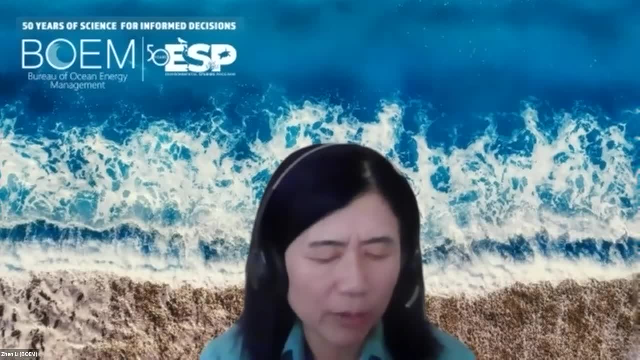 Recently, the Arctic has experienced rapid environmental changes, Such as decline of sea ice content and increase of ocean acidification, which could impact Alaska's blue economy. The effort to build Alaska's blue economy includes mariculture, using marine microalgae to produce biofuels. In this session, two experts will present perspectives on Alaska's blue economy and microalgae research inspiring. 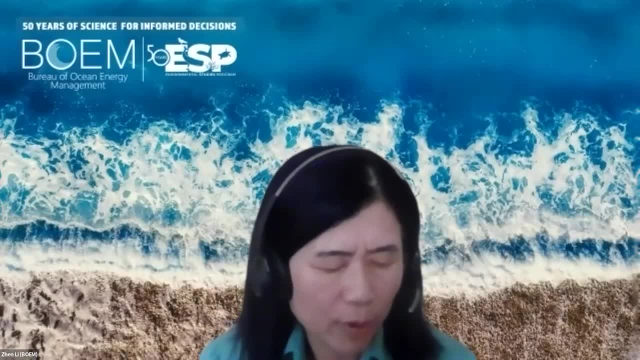 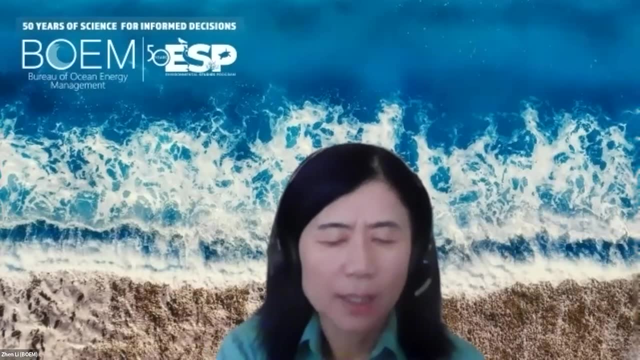 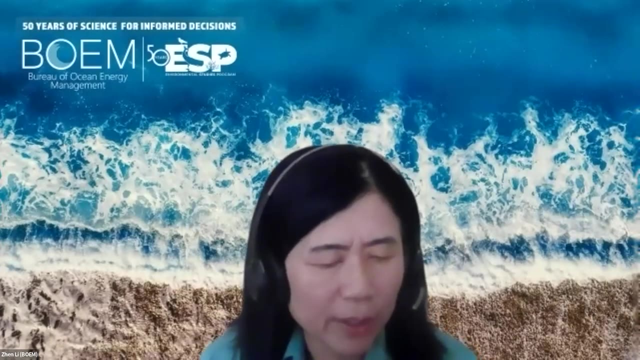 novel energy research. We are very lucky to have invited two very distinguished scientists to give presentation. At the very last minute we switch the sequence of presentation Now we have. our first speaker is going to be Michael Steckle, Professor of University of Alaska, Southeast. He will talk about marine culture of sugar cap as a scalable model for offshore. 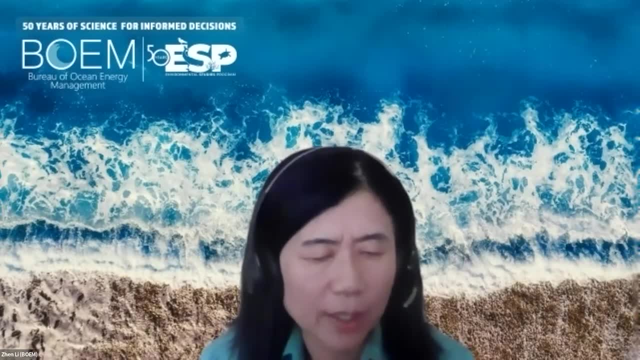 marine culture of sugar cap as a scalable model for offshore marine culture of sugar cap: as a scalable model for offshore cultivation. The second speaker is Justin Steinberg from the University of Alaska, Fairbanks, and he's a Director of Alaska Blue Economy Center. He will talk about the applied blue economy, developing industry and community engagement in Alaska. 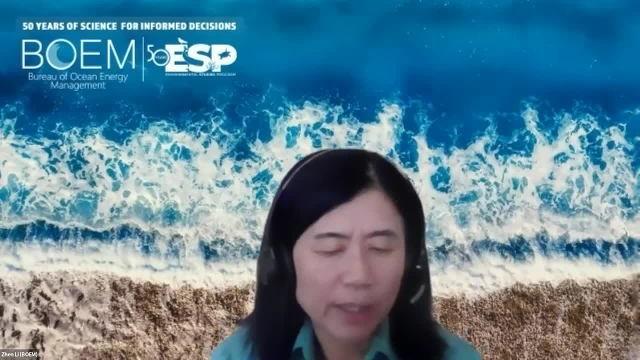 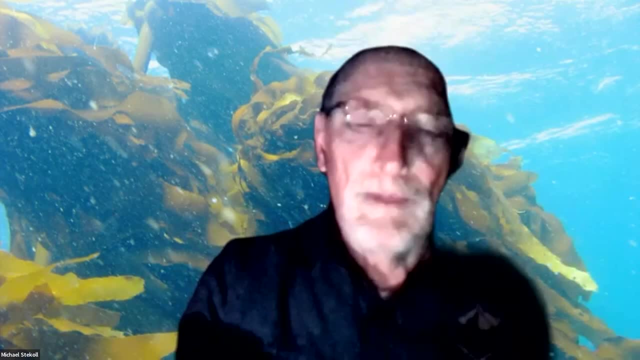 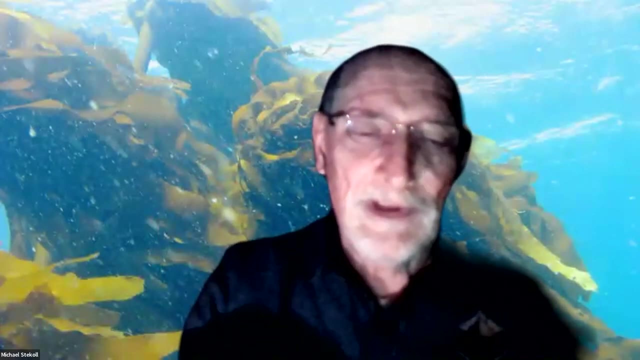 Now let's welcome our first speaker, Professor Michael Steckle. The floor is yours. Now let's welcome our first speaker, Professor Michael Steckle. The floor is yours. Okay, thank you. So I am an actual professor emeritus at the University of Alaska and I'm now associated with Fairbanks- not Southeast, but it's in the same place, still in Juneau. 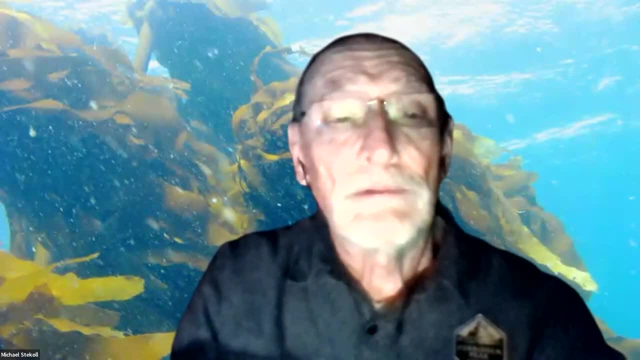 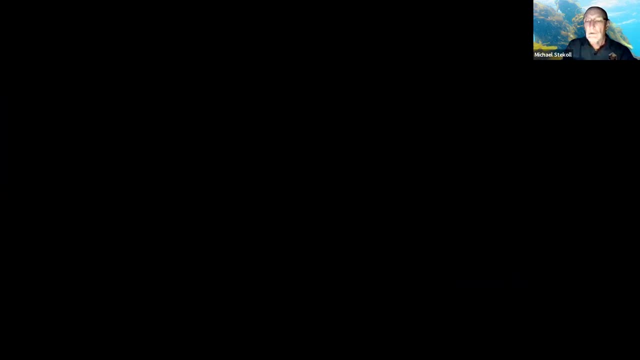 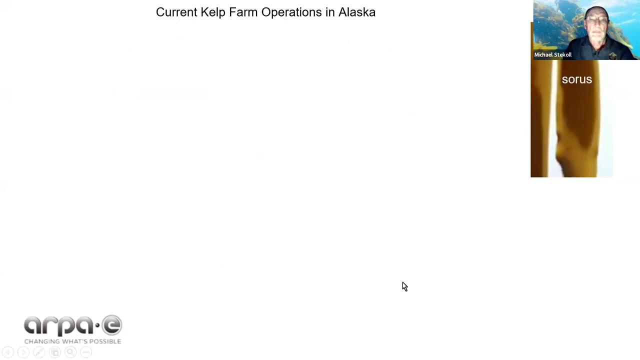 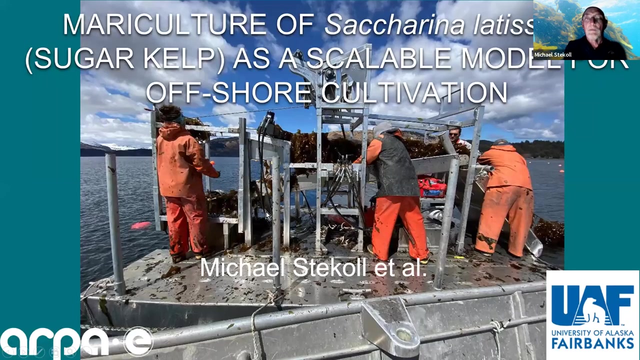 So I'll share my screen here. Okay, Well, it was working before, wasn't it? There we go, Okay. So, as mentioned, we're going to talk about our work that we've done in Alaska on the miracles of sugar kelp. 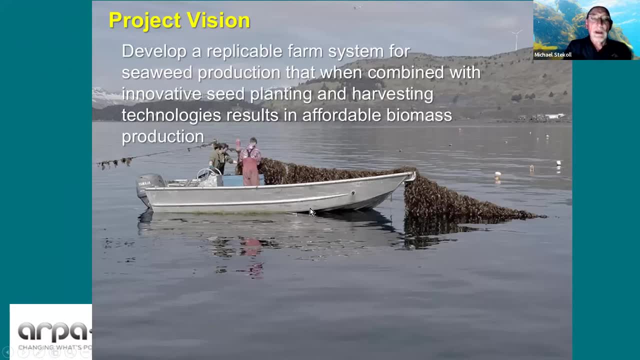 And the vision basically is to develop a replicable farm system for seaweed production that, when combined with innovative seed planning and harvesting technologies, results in affordable biomass production. So the goal here with RPE funding Is to is to look at the feasibility of large scale seaweed culture that might be used for biofuel are used in some energy capacity. 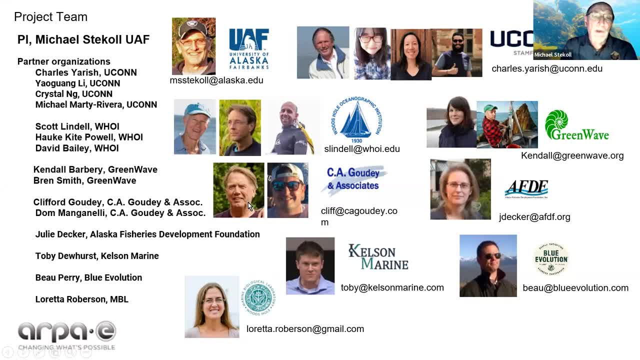 This project is has a lot of team, a lot of people on our team- sorry, Aside from myself- there's Charlie Yerch's group in the University of Connecticut, Scott Lindell's group from HUI, Kendall Barberry from Green Wave. 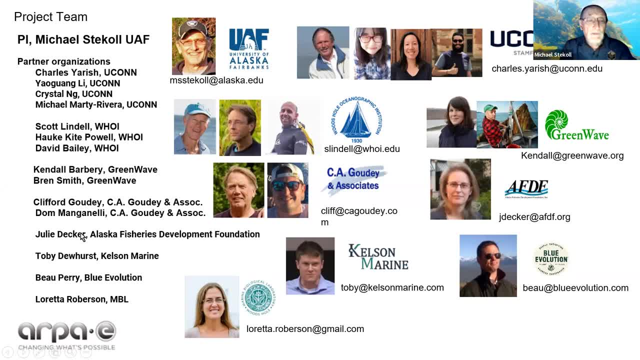 Cliff Gowdy, our engineers, Julie Decker from Alaska Fisheries Development Foundation, Toby Dewhurst from Kelston, Marine Beau Perry of Blue Evolution, who's our- our private partner, business- sorry, industry partner. And Loretta Robertson from Marine Biological Lab. 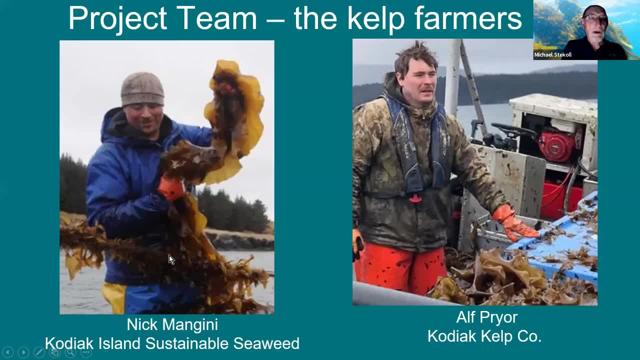 And, of course, a lot of other people that we hire and are. the main people here are Nick Mangini, who's our seaweed person, who grows seaweed in Kodiak, and also Alf Pryor, also a seaweed farmer in Kodiak. 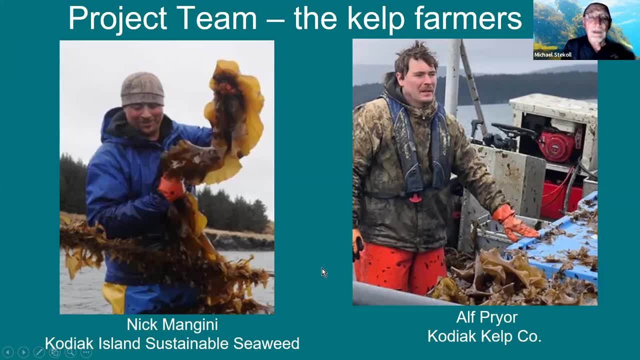 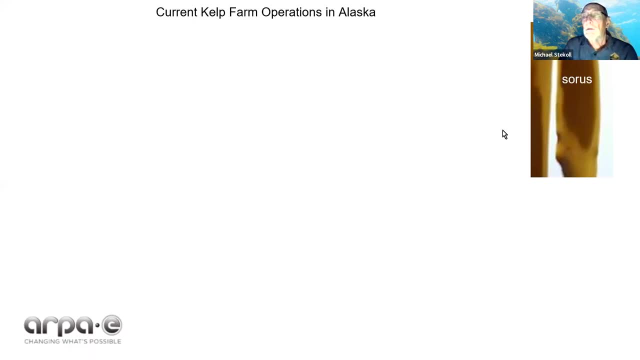 Without who, Without who, Without who sold these two people? these two people, nothing would happen. So first I want to talk about the. let's get some stuff out of the way so I can see myself the process of of growing seaweeds- at least these kelps here. 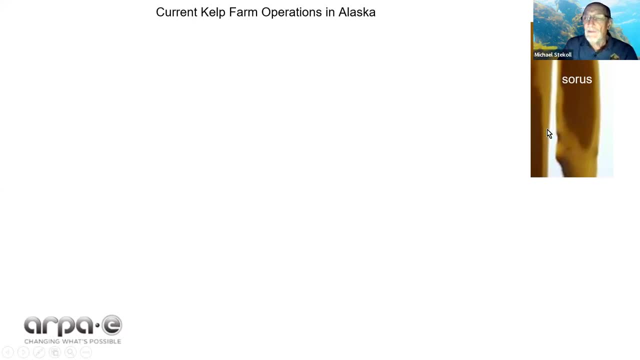 So first we find a fertile plant in the field that has a fertile area called a saurus. We release spores from this, spores that kind of like this. they swim around and they settle out And then And then grow into an alternate, one end gametophyte phase where there's females and males. 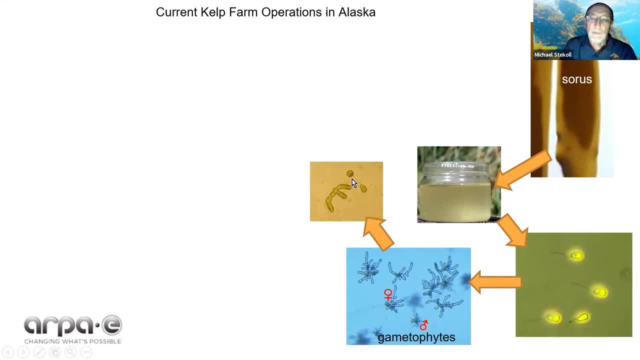 And, under certain conditions, they'll become fertile, making this as an example of female egg sperm, and will grow into little baby plants. In the actual hatchery itself, or so-called hatchery, we take from the spores and we settle them on. 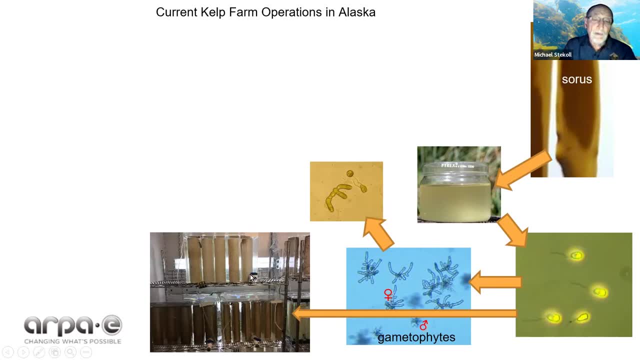 On String that are wrapped around these spores in in tanks. we give them nutrients, let them grow for six or seven weeks until they look like this on the string. So these are baby plants. now, now these are sporophytes. 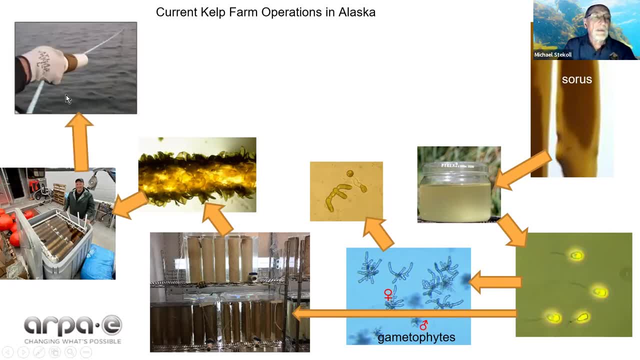 We take these out to the field in the in the cylinders, wrap them around string. these are. these are long line out plantings and we put these in a structure similar to this, where the plants are going to be growing, hanging about three meters under the surface. 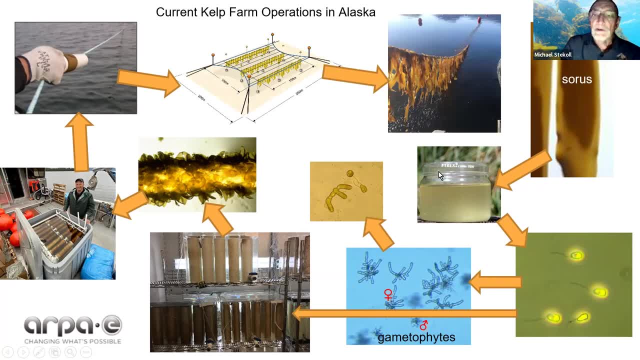 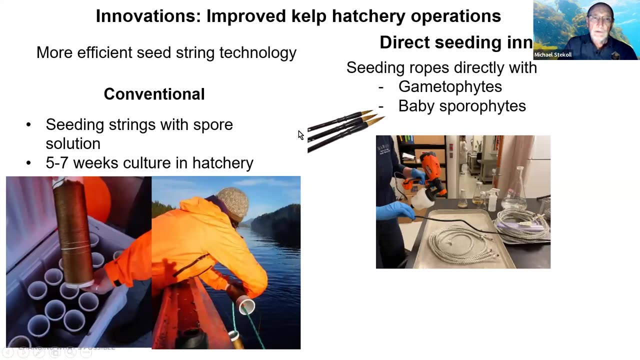 And then The new season positioning The product. These are outplanted in the fall, usually around November, and they're harvested in usually May or June. This area here is what we call it The hatchery, One of the things that we try to improve the process. 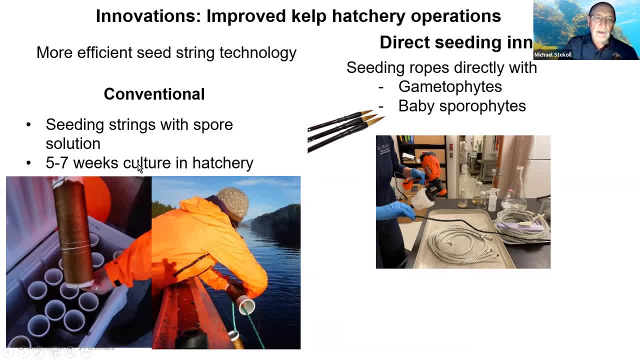 So This is our, our hatchery improvement process. So them for five to seven weeks. culture and hatchery in modified medium: uh, direct seeding is a new innovation that's being applied by a lot of different people now, and we're trying it here. 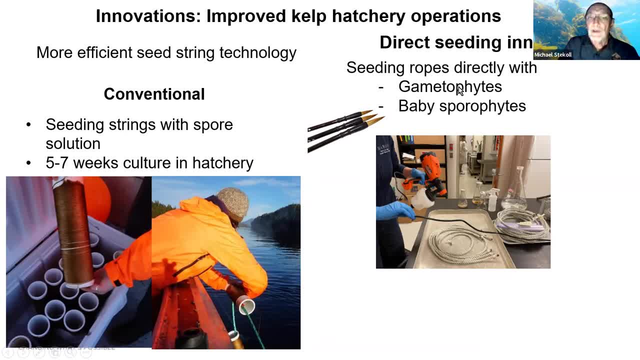 in alaska was seeding ropes directly with gametophytes or with baby sporophytes and basically this would give us no need to gather parent plants each year because we could keep these gametophytes growing and keep them growing, uh, as gametophytes and not get fertile for a long time. 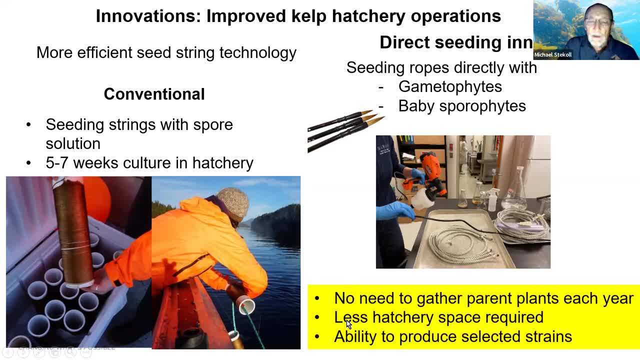 if you keep them under red light or or without iron? uh, there's. so there's less hatchery space required because you can, instead of having hundreds or even thousands of these schools, you just have a couple of flasks and we can produce selected strains with this, because 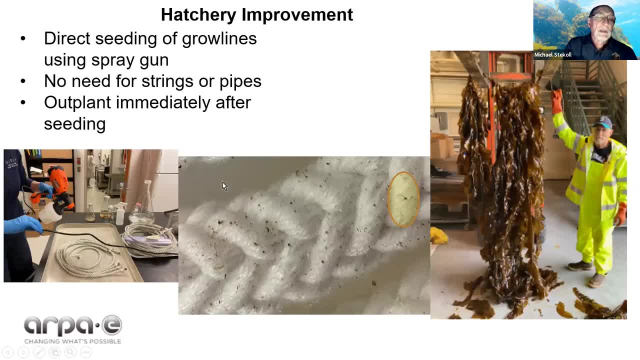 everything can be done from clones. so in kodiak we did some direct spraying. basically we take a gametophyte solution and spray it on these, these ropes here and uh. you can see in the center picture here. this is: these little dots are gametophytes and this little thing. 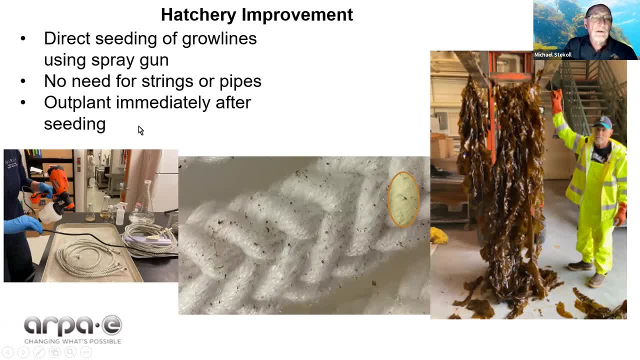 circle. here is a baby sporophyte, a baby blade- so we don't use strings or pipes- and after spraying these, we put them in the cold room for a couple hours and then took them out to the ocean, out planted them and we got this kind of result here. so, uh, it can work and we need to refine the 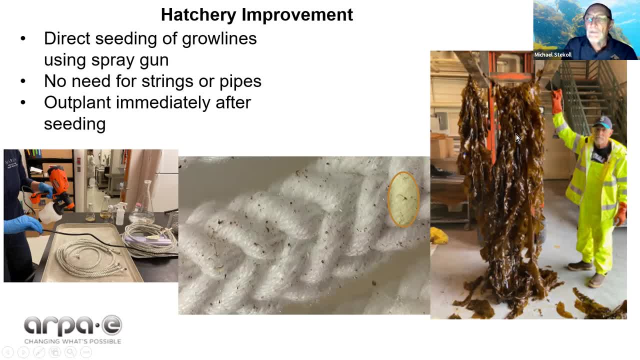 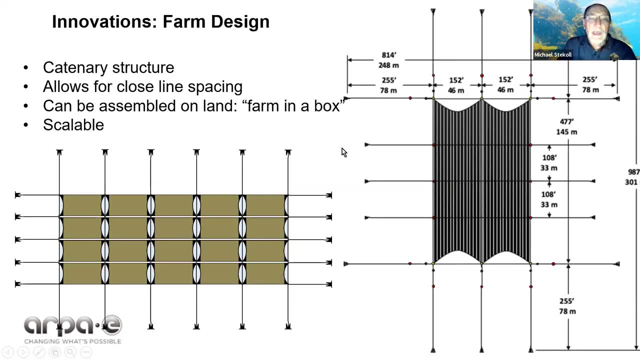 process more and figure out how to might automate it, but uh, we have a lot of positive feelings about spraying. the other innovation that we are doing is a catenary structure type farm. this has been developed by cliff gaudy of tandocian and his colleagues. basically, the catenary system, which 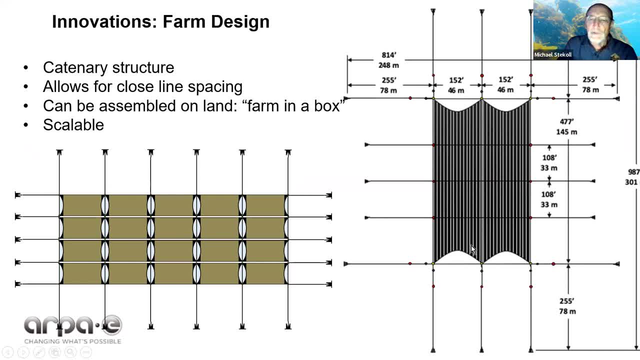 is these catenaries? here uh is chosen because if the lines are properly measured, then the lines can be very close together with under tension and they won't cross over each other and, like you would have if you had, say, individual lines each held by anchors. so this catenary system has got a lot of promise in keeping uh, in allowing us to grow. 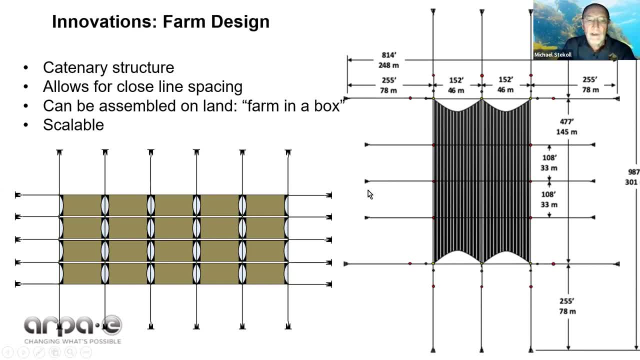 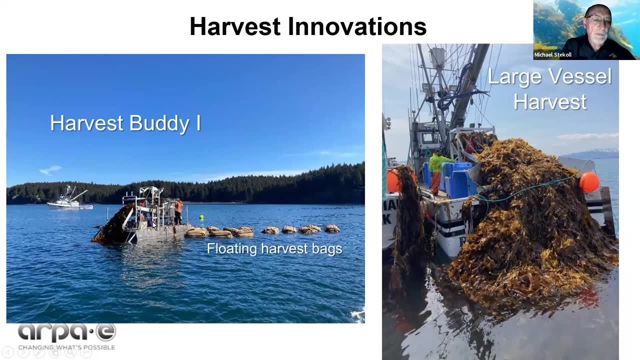 large amounts of seaweed in a small, smaller space and the also advantages that shown here on the left. you can put these things together so it's it's scalable in that sense. another innovation that we have tried is a special built harvest vessel here called the harvest buddy. that will 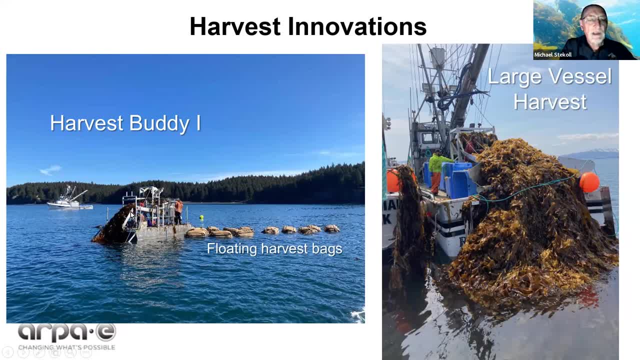 pull up this, the lines. you can see the lines coming up here on the left side. it cuts the plants off and drops them into these bags here, flowing here. the bags are, are closed up and they gang together and they float away and even though these plants are very heavy, these bags float for a long time. so 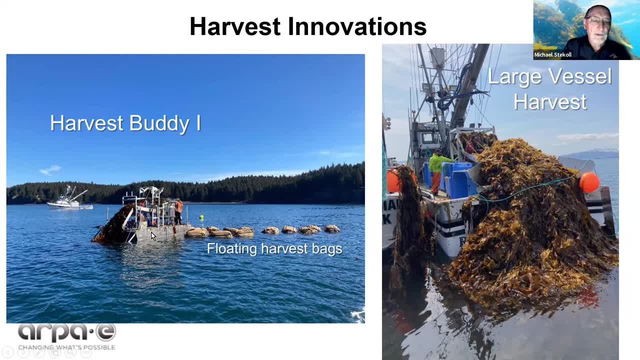 you don't need a special boat here to to hold all the the harvest, they can just float away, not too far of course, and then the uh tender here can come over at leisure, basically, and pick up the bags and take them back to court. and the other thing we tried was, uh, having a larger vessel harvest, and here's an example of 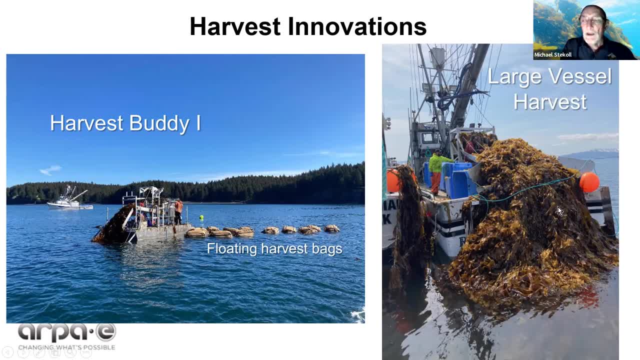 a larger vessel pulling in five lines at once. uh, it's a turned out to be a basically overwhelming biomass to try to handle. so, uh, this last year we we bought, we changed this to one line and it seems to work a little bit better. trying to get things going with that. 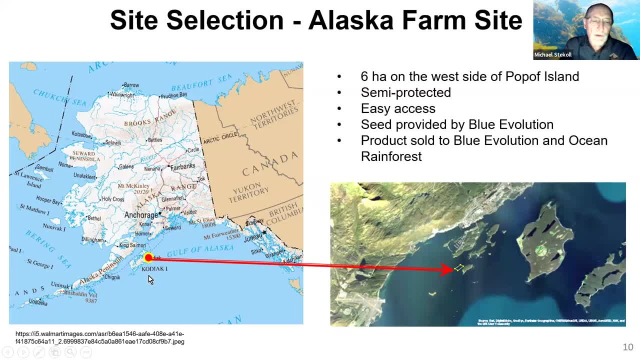 our farm itself is in Kodiak, as I mentioned here. Kodiak, there, and here's where the farm site is, over in the right, this little area here, um, semi-protected, easy access. it was something that was already, uh uh, leased by Nick Mangini, so we had a ready, ready-made farm, basically to work to. 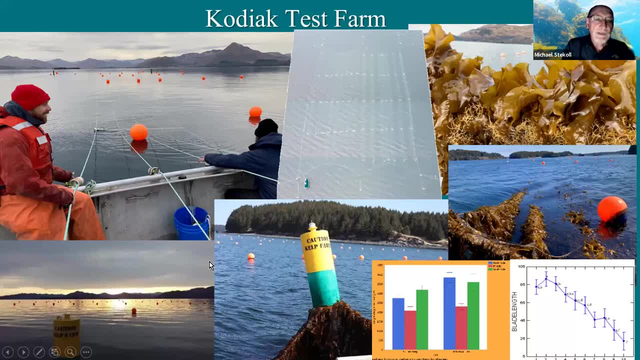 work with and here's some pictures of the farm where the past few years. here's, uh, our seeding procedure. here you can see the cylinders. here with a string going out. there we can see five lines at once. here's an overview of the farm itself. some of the product on the right side here. 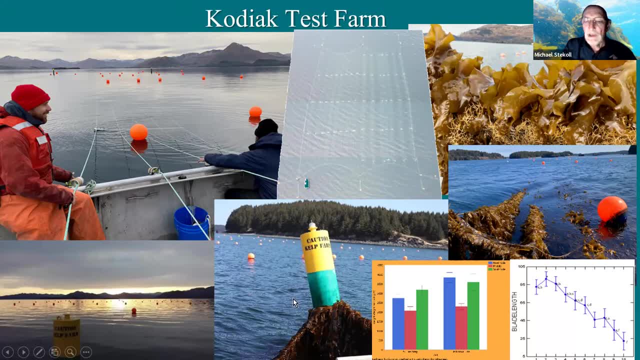 uh, this is our farm site in the middle. a couple of pictures on the left and then on on the right. here it's a couple of data points showing that on this right hand side, we show that the best growth of growing these things with experiments- so some experiments- it shows that the best growth is. 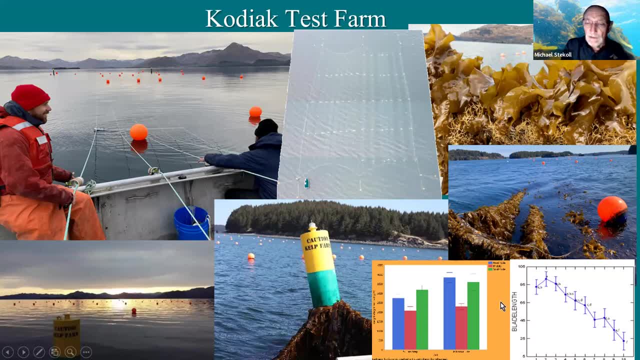 between one and four meters deep, and the picture on the left here shows that the growth at the end of the season for our first year showed that the lines in the middle of the farm were to be run. these areas here, uh, sagged quite a bit and therefore the down below this, this optimal depth, and the lines in the 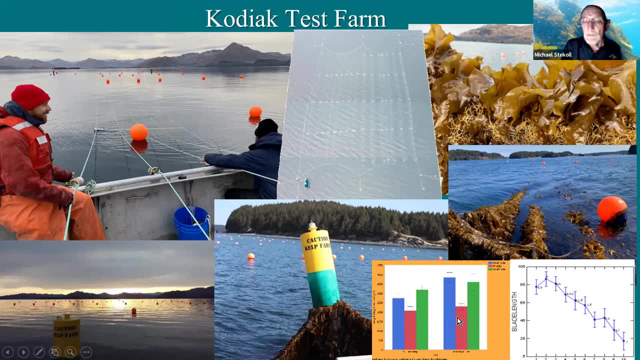 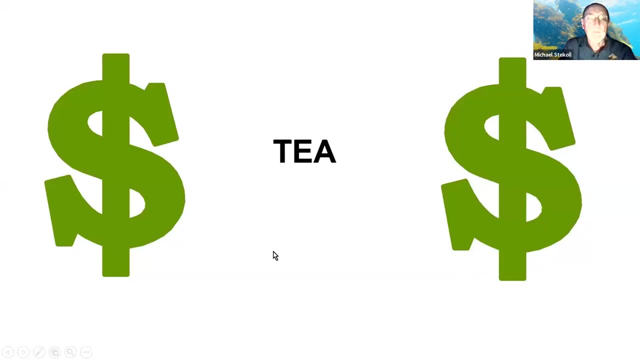 middle or the plants in the middle then grew much smaller. so we changed that the next couple of years by adding flotation, which we didn't have the first year, and aside from other problems, we just need to be on the right track and try to get large amounts in a smaller space. we also do some work with TEA or 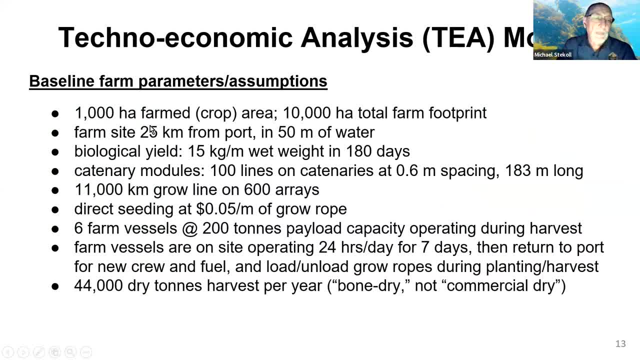 technical economic analysis. so our TA person from Woodsoil made some assumptions that this is what would happen if we, if this could be done for biofuels, a thousand hectare farm, 1000 hectares total farm print because the the scope of the anchors, the farm sites, about 25. 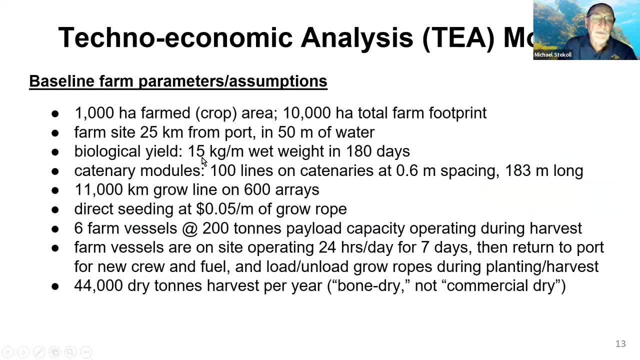 kilometers from port. at 50 meters of water we get- we're assuming- 15 kilograms per meter wet weight in 180 days. we use catenary modules: 11 000 kilometers of grow line, 600 different arrays. we use direct seeding instead of using those strings. six foreign vessels at 200 tons payload. 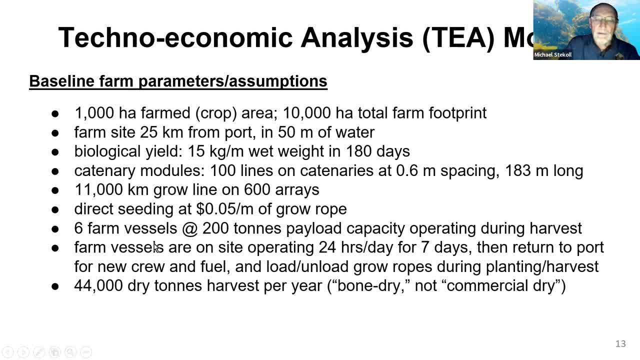 capacity operating during the harvest. foreign vessels are on site 24 hours a day, seven days, then return for new crew, and so on. 44 000 dry tons harvest per year, and so at the end this is a big spreadsheet figuring out how much everything would cost. but look over here on the right. this: 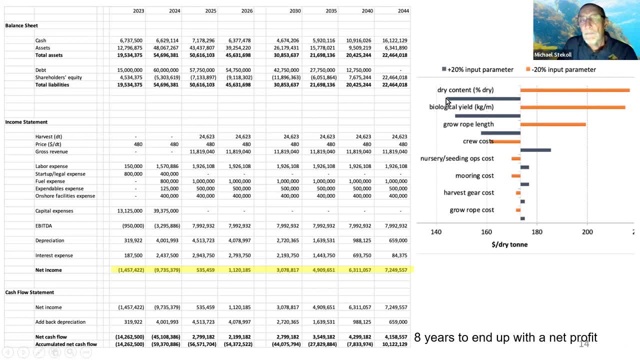 tornado diagram shows that the cost depends on, mainly depends on, the dry content of the plants, which is about 10 percent. if you could increase that, then you could increase your, your yield and your profit, and also just a straight yield kilograms per meter online, could. it would also. 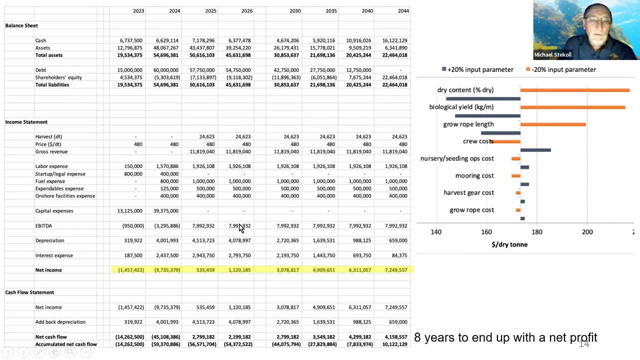 if we could increase, that would also decrease the cost quite a bit. but down here at the end here, so it's net income. so we lose money for the first two years, uh, in terms of capital expense and so on, and then third year, start making a profit for that year and continue to make profit out of that if 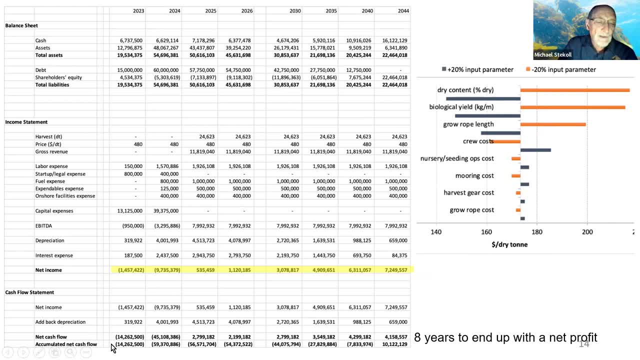 everything is sold, of course. so down at the very bottom here is a accumulated cash flow and we see that we're we're in the hole for eight years till we finally have a net profit. so with all those assumptions, it still takes eight years to to make a profit with this sort of sort of very large farm. this would be a large farm on. 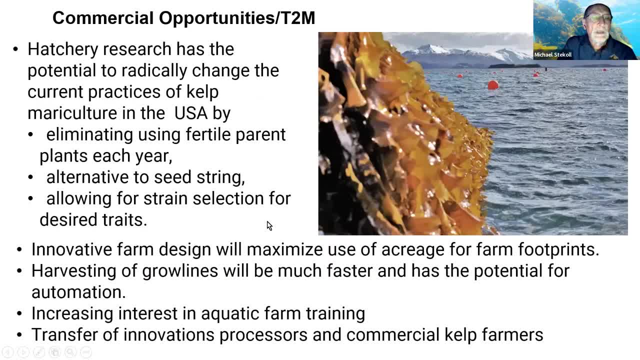 the outer, off the outer coast. so our hatchery research has potential to radically change the current practices of kelp because we eliminate using fertile plant parents each year, parent plants. it's an alternative. seed string allows for strain selection for desired traits. our innovative farm design, we think, will maximize use of acreage and farm footprints. 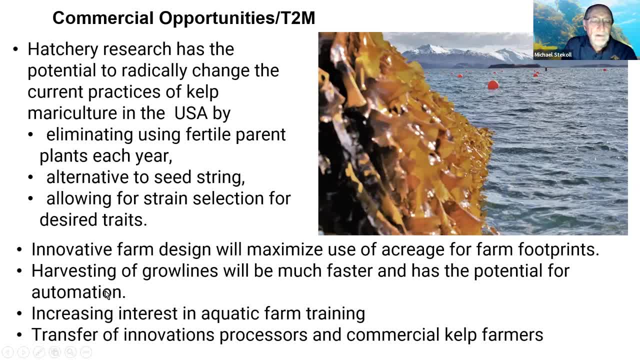 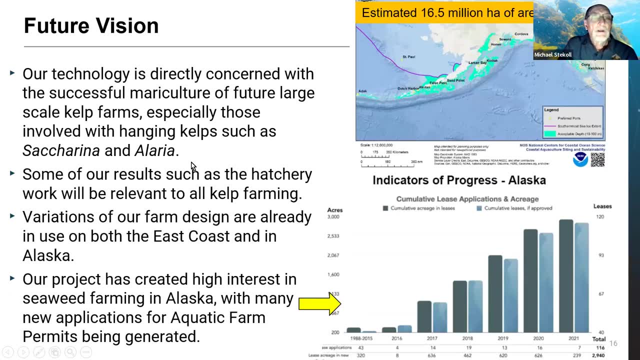 harvesting grow lines will be much faster as potential for automation. all the stuff that we've done has increased interest in aquatic farm training and aquatic farms in Alaska, and transfer of our innovations processors and commercial co-farmers is already happening. so our technology is directly concerned with excessive agriculture of future large-scale farms. 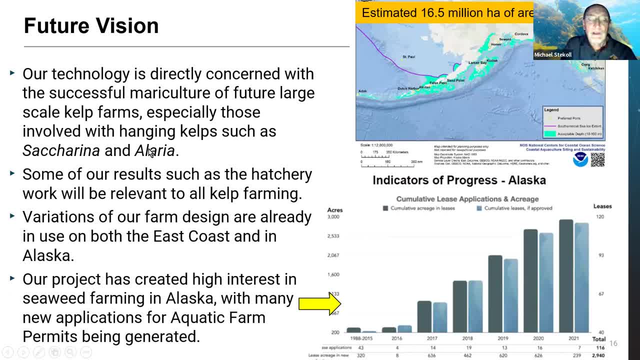 especially those involved with- and a lot of places are in California, for example- are doing bull kelp and and- uh, giant kelp, which are floating cups, and the technology we have here may not work with that. some of our results, such as the hatchery work, will be relevant to all kelp farming. variations of our farm design are already. 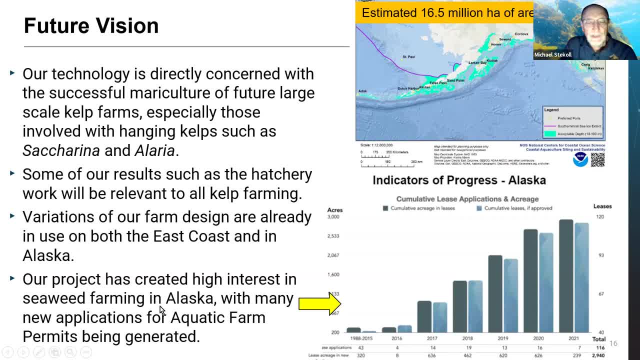 being used on the east coast in Alaska and our projects create a lot of interest in Alaska in seaweed farming and aquatic farming in general. and on the right here shows uh the uh number of new plants that are being processed in Alaska. so it's we're getting kind of an exponential rise in. 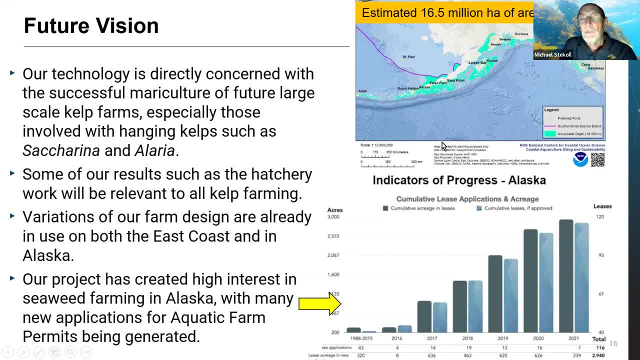 permits. of course this can't keep going because it's only so much land. but up here in the diagram up here uh shows what we think might be the potential areas offshore for growing uh seaweeds in Alaska. so we have considerable area and several problems, especially uh areas out here. if uh 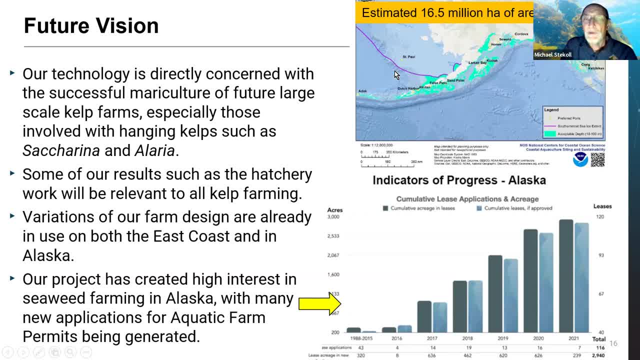 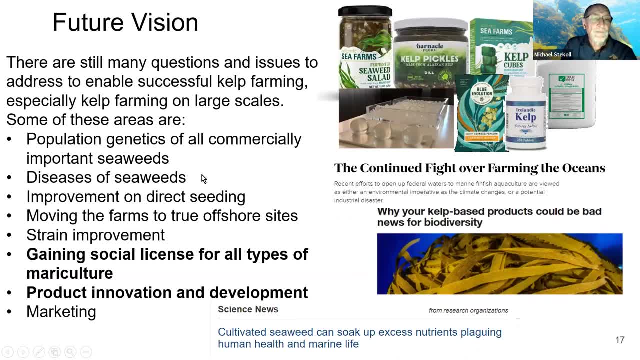 climate change happens enough that we becomes ice free, that has a lot of potential for Alaska. that's- I guess that's good news, sort of so. so many questions and issues to address for successful farming. here one is: we need to know about population genetics of all commercially important seaweeds. this is important in order to 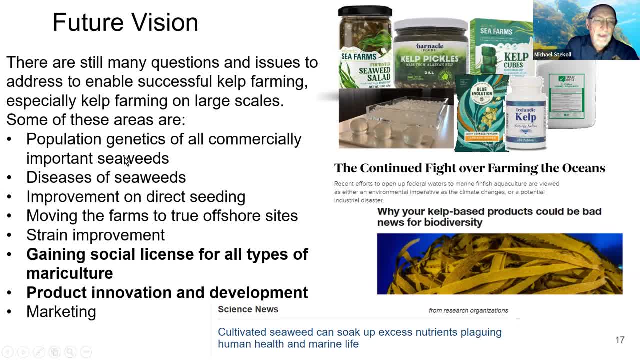 not cause uh harm by mariculture by changing genetic composition of a nearby natural beds. we need to know about diseases of seaweeds and how to treat them. we need to improve that direct seeding process. we need to figure out how to actually move Farms to true offshore sites. right now we're not there. 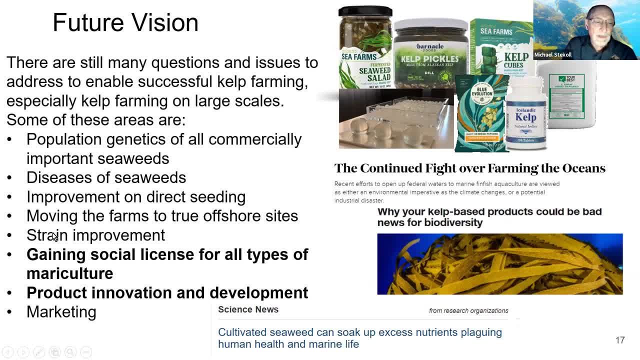 um, it'd be good if we could do strain improvements- not allowed in Alaska, but it's other places. but some more important things are gaining social license for all types of Mariculture, because that's a big barrier to Mariculture and a lot of states in the United States. 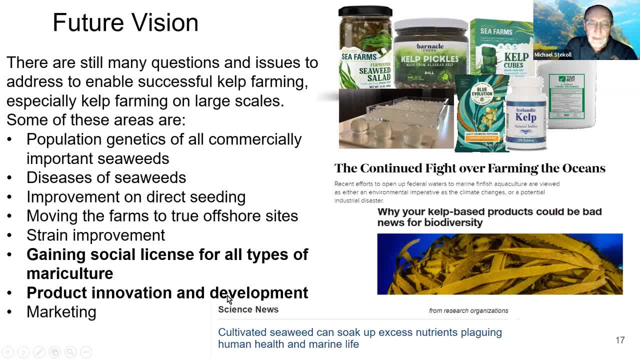 and product innovation development is very important because until we have huge farms that can make enough biomass for biofuels, we need to make these smaller farms profitable, and they only can be profitable if they have some type of product they can actually sell, and that also false marketing. 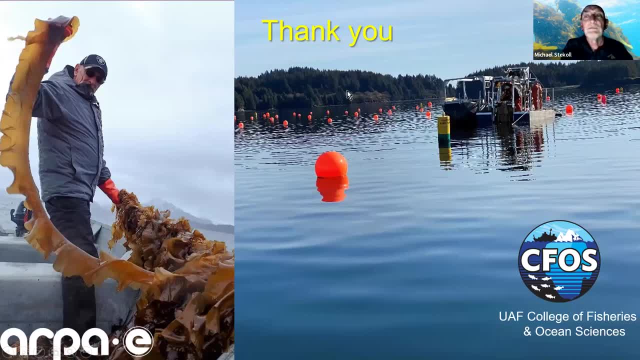 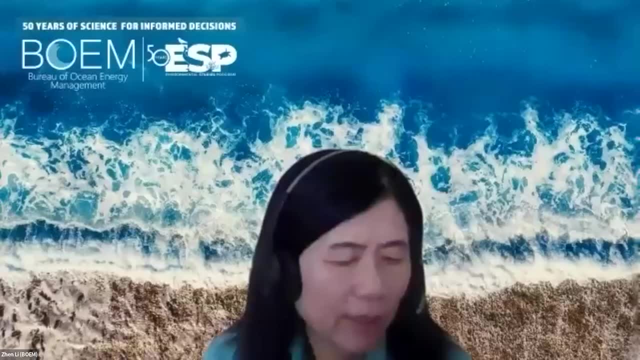 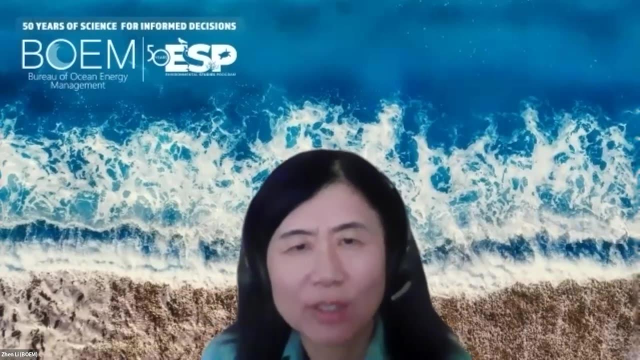 so that's all I have to say right now. thank you very much for listening. yeah, thank you, Michael, for your presentation. we have uh about the um. yeah, we still have maybe like people can maybe hold on the question until that second speaker give a presentation. You're right on time. 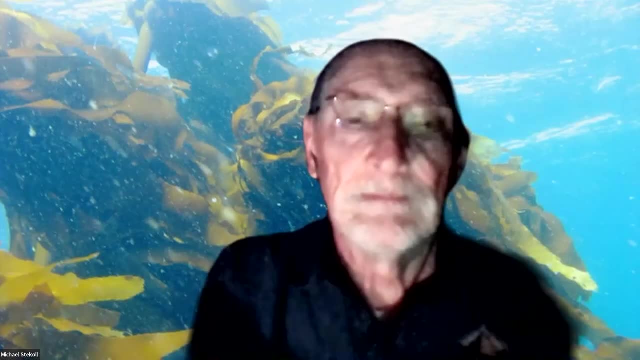 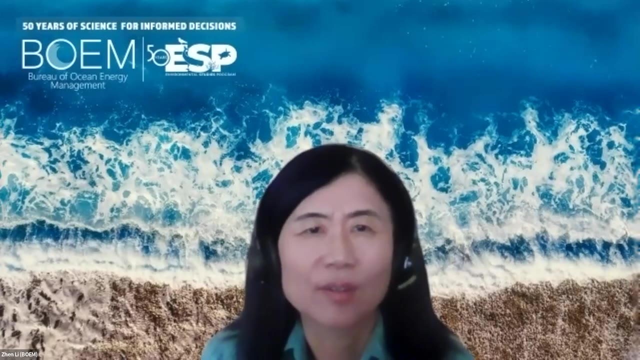 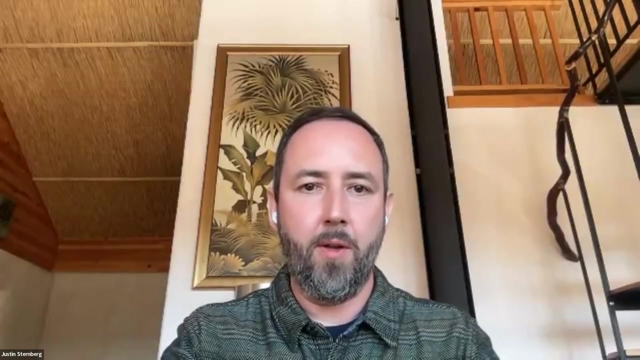 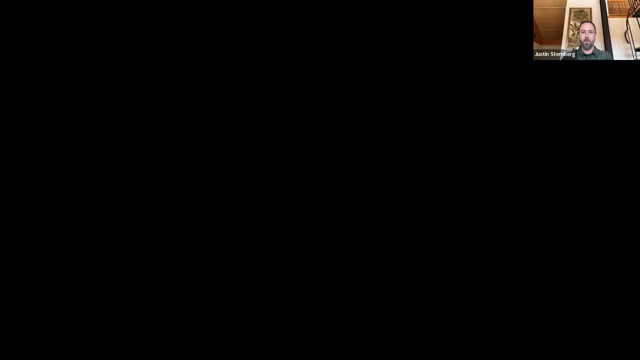 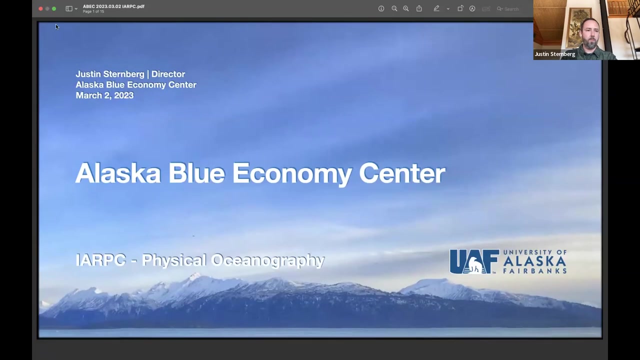 Thank you so much. Okay, Now let's welcome our second speaker, Justin Sternberg, to present. Hello everyone, Thanks for having me here, Grateful for the opportunity to present to you all. Can everybody see that? Yep, Great Thanks. 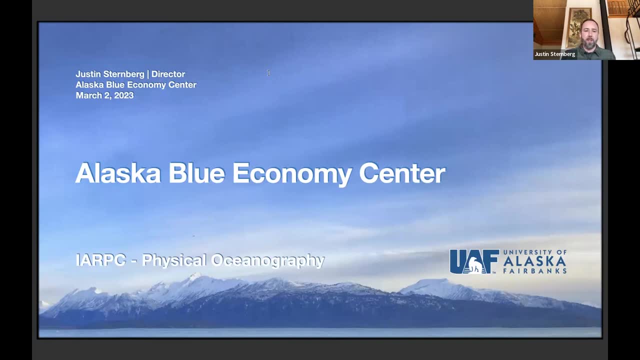 So my name is Justin Sternberg. I'm the director of the Alaska Blue Economy Center at the University of Alaska, Fairbanks, And I'm going to be talking about the center's role at the university and our partnerships with communities and industry partners. 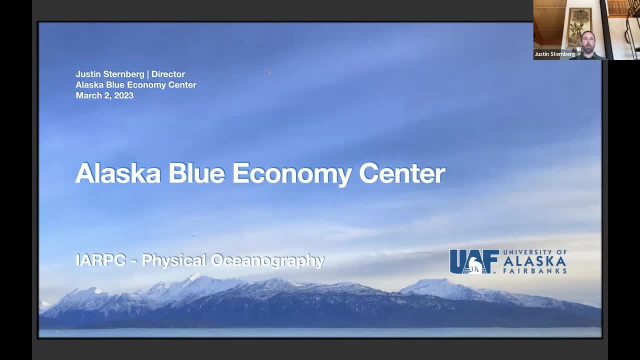 And some of the tasks that we're doing within the university with our internal partners to address opportunities for Alaska's economy in the ocean and water related sectors. I am not a research scientist. I have a background in business in the private sector, initially working in renewable energy and energy efficiency. 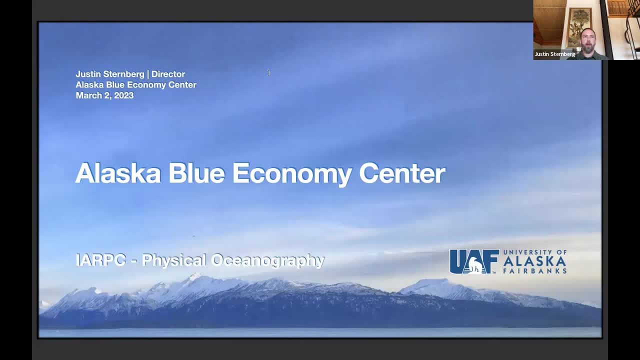 I've worked in Alaska since 1997, and I got into the ocean related space in 2014 with working with a colleague from my MBA program, Bo Perry, who Michael mentioned in the last slides is the founder of Blue Evolution. And in 2014, we set up a public private partnership with Mike and his lab to develop commercial seaweed mariculture in the state, which had never been done before. 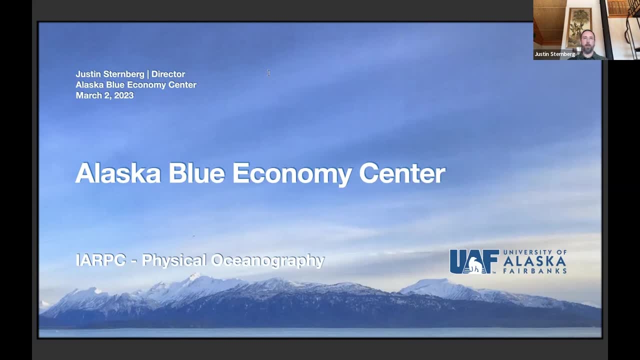 And I ended up working with the Department of Fish and Game on the permitting protocols- which are largely still in place as they were as as we develop them in partnership with the state- and then also permitted the first commercial hatcheries and farms, One of which was with Nick Mangini, who was in the slides that Michael showed. 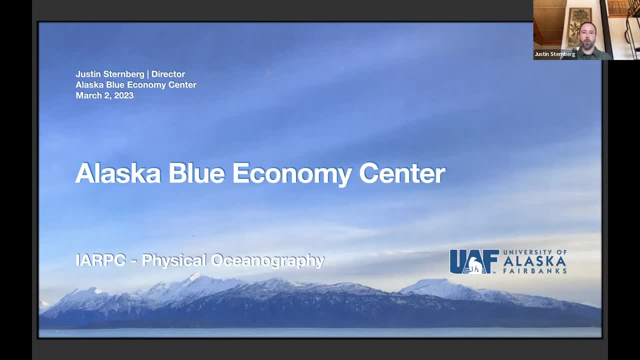 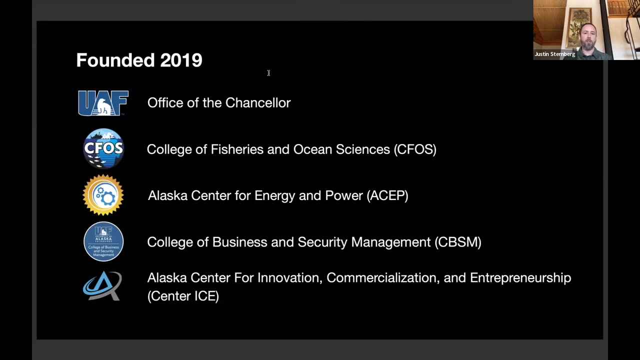 Subsequent to that, I worked with the Alaska Ocean Cluster developing entrepreneurship in ocean related industries, and then joined the university in my current role in the summer of 2021.. So the Alaska Blue Economy Center was first stood up in 2019 at the direction of the Office of the Chancellor. 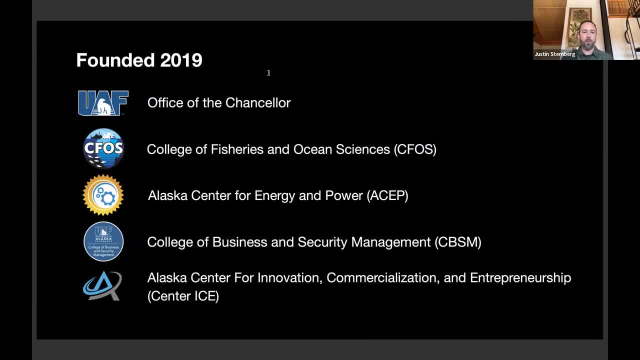 So the Alaska Blue Economy Center was first stood up in 2019 at the direction of the Office of the Chancellor, And then I joined the University of Alaska in 2020, which included Dan White and included four different units within the university. They came together recognizing that there was an opportunity for the university to engage further with ocean based industries and recognizing the value of the ocean and the river systems to the state's economy. 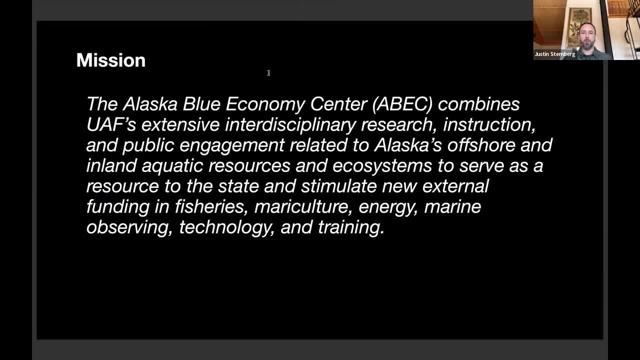 Our mission is to combine UAS extensive interdisciplinary research, instruction and public engagement related to Alaska's offshore and inland aquatic resources, resources and ecosystems to serve as a resource to the state and stimulate new external funding in fisheries, mariculture, energy, marine observing, technology and training. 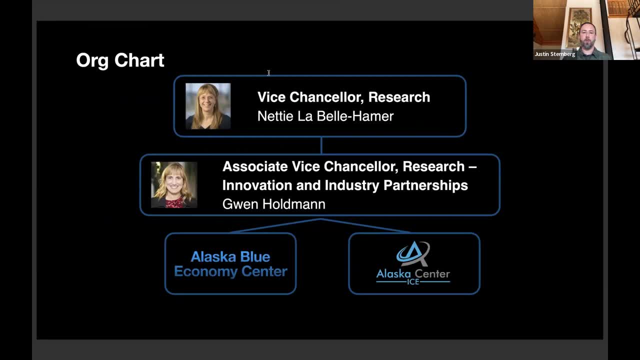 We're located within the Office of the Vice Chancellor for Research, and recently there was a change where Gwen Holdman, who was previously the founding director of the Alaska Center for Energy and Power, moved over to a new role within that office as the Associate. 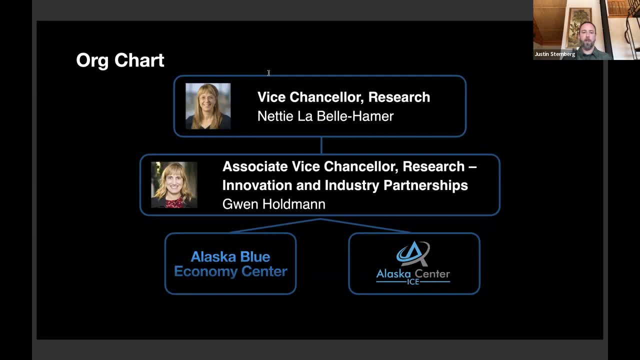 Vice Chancellor for Innovation and Industry Partnerships, Gwen's been building out this ecosystem for some time. In addition to setting up ASEP, the Alaska Center for Energy and Power, she also was one of the co-founders of Alaska Center ICE, which stands for Innovation Commercialization. 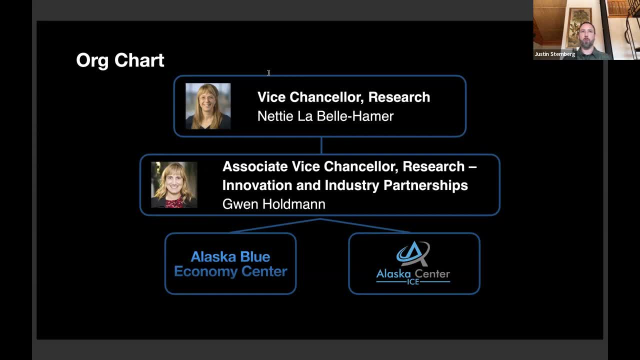 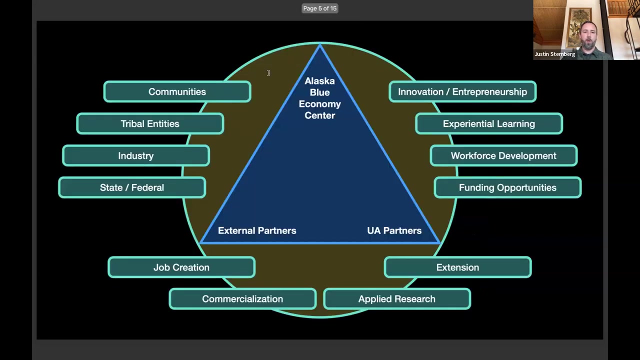 and Entrepreneurship that leads entrepreneurship activities in the university, as well as patents and intellectual property. The Alaska Blue Economy Center is the newest addition and we came over to the Vice Chancellor's office when Gwen's role was initiated last May. So we partner both internally within the university and externally, and these are some of our. 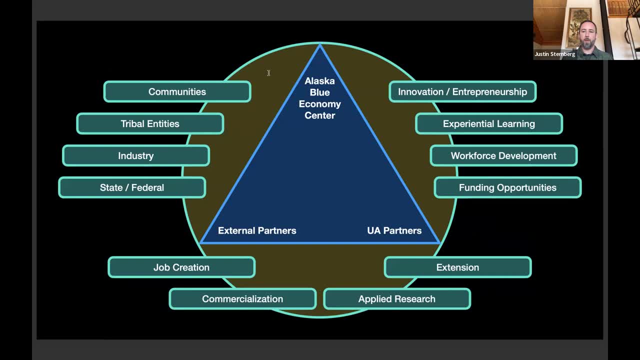 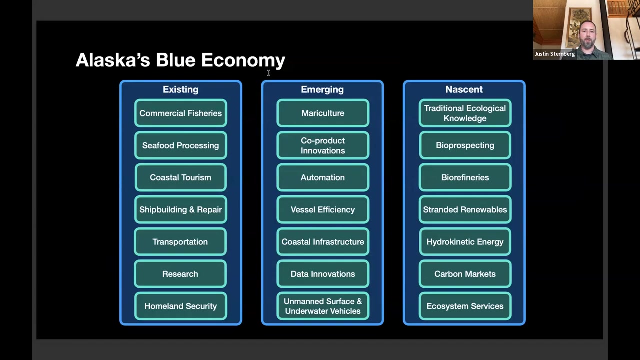 external partners in the upper left, Our roles within the university and the upper right, And with both our internal and external partners, focused on job creation, commercialization, applied research and extension. Alaska's blue economy is already quite impressive. We have some of the largest fisheries in the world, more coastline than the rest of the 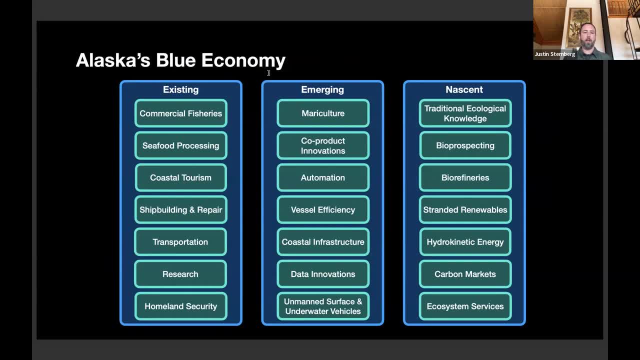 United States combined, We have the largest naturally occurring kelp beds in the world and some of the best kelp-growing habitat in the world. This slide outlines some of the existing areas that are fully developed and go back, in some cases, hundreds of years. 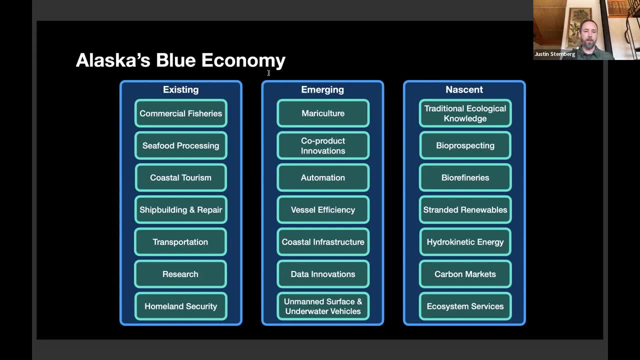 The fisheries I mentioned. we recognize seafood processing as being distinct from that. And then coastal tourism is also a huge contributor to the state's economy. Shipbuilding and repair is a smaller component but shows lots of promise for the future. And then we have a lot of other areas that we're working on. 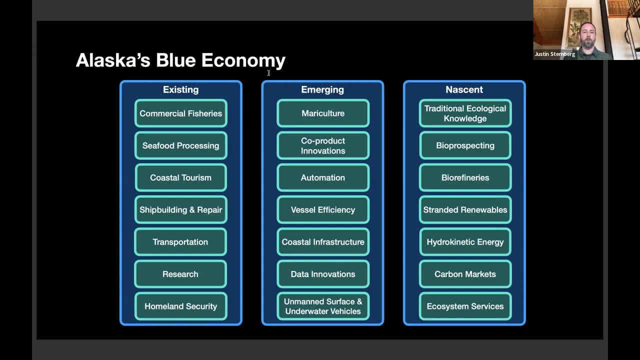 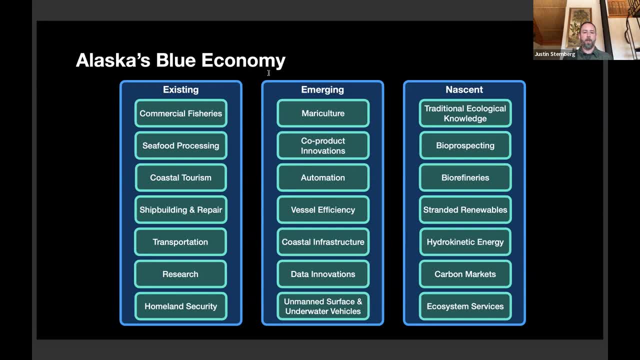 We have a lot of other areas that we're working on, But a lot of it is expanded And when I think of the хватfish, we're talking about size and size and kind of the size of fish we're cooking. 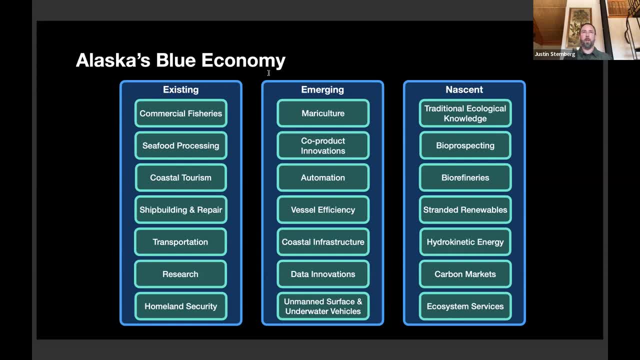 or the size of the size of the fish we're cooking, and that's on other areas that we're focusing on. So that's a big part of the economy. The economy is deployed to develop value-added products. In some cases, these products can be more valuable than the 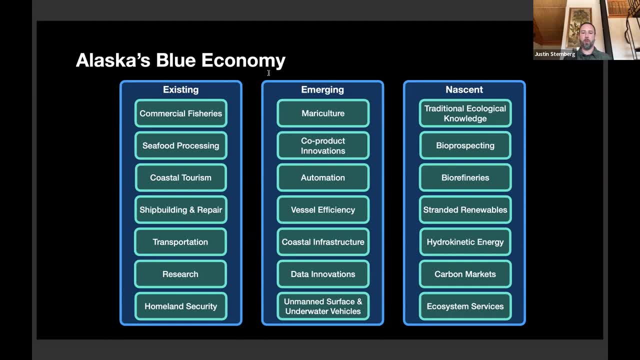 protein from the fish. There's an increasing need for automation, which was made clear during the pandemic. Getting people in and out of Alaska can be really challenging, especially to very remote locations, And some of the jobs that could be automated are actually better done by machines. They're very challenging. There's not enough workers. Typically, the 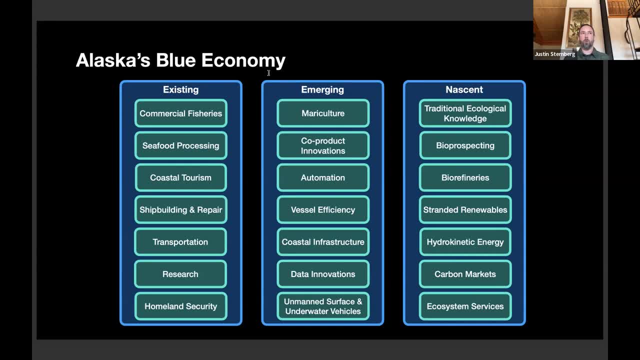 industry is importing workers using H-1B visas from the Philippines, And so there's a challenge there and a need for automation. Vessel efficiency and energy in general for the seafood industry is critical, as is the infrastructure that's needed around the state. There's very few ports. 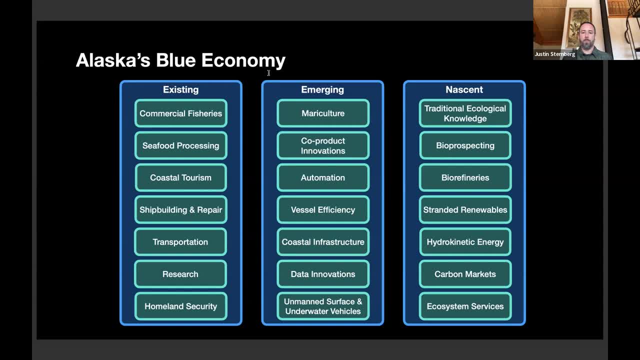 in Western Alaska, for example. There's very few ports in Western Alaska, for example. There's very few ports in Western Alaska, for example, Deepwater ports. And another area is data innovations, as we're able to go into the ocean at much lower costs and with better. 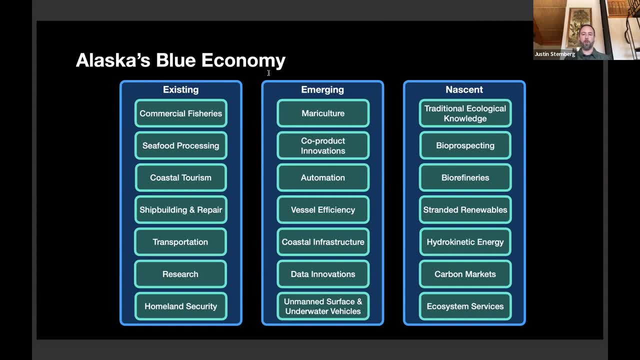 technologies in ways that we were never able to before. We're starting to pull out increasing amounts of large data sets that are requiring data specialists. There's also a whole host of nascent industries that are just kind of, in some cases, not even getting started, but 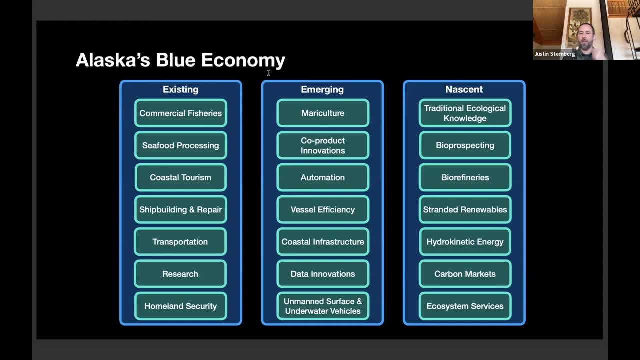 waiting to be started. Traditional ecological knowledge is something that's increasingly being recognized through research as an important component of economic development. and engagement with Alaska Native communities, recognizing the value of their knowledge and what it can bring and the potential for creating economic development in their communities. 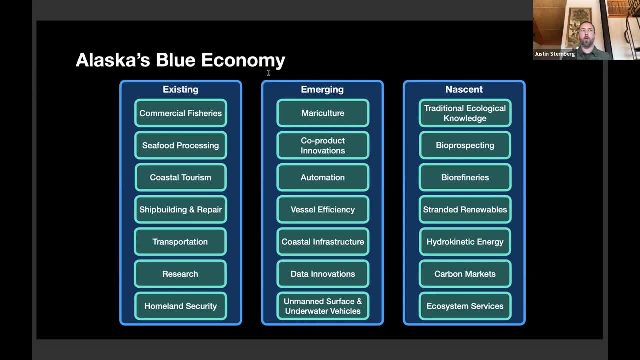 Bioprospecting: We have some of the largest cold water ecosystems. Bioprospecting: We have some of the largest cold water ecosystems in the world and they're largely unexplored or underexplored. And then carbon markets, skipping down a few, there is. 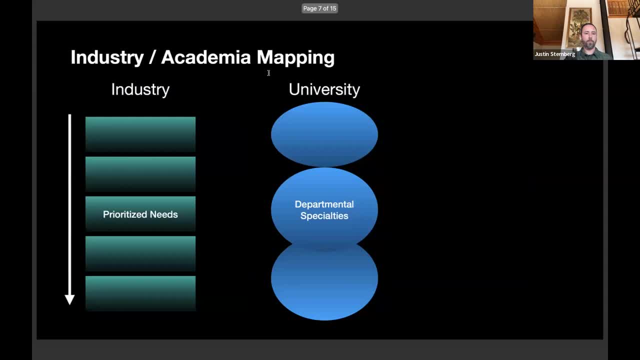 something that was recently identified that I'll talk about here a little further. One of the primary activities that we're doing is working with industry and within the university to map out where the industry's needs are, where their challenges are, what they see as solutions. 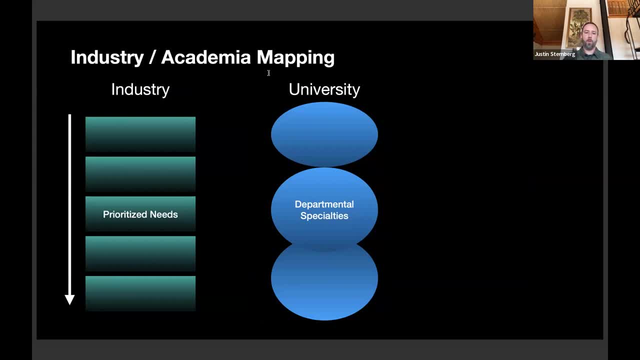 and what they're looking for in the future. And then we're also working with the industry to map out where the industry's needs are, where their challenges are, what they see as solutions, and then mapping that to the university's specialties. So initially it's often interdisciplinary. I've got the lower two departmental specialties overlapping. In some cases the departments work closely together and other times they're working more in parallel and there's not a lot of communication between the various departments across units. 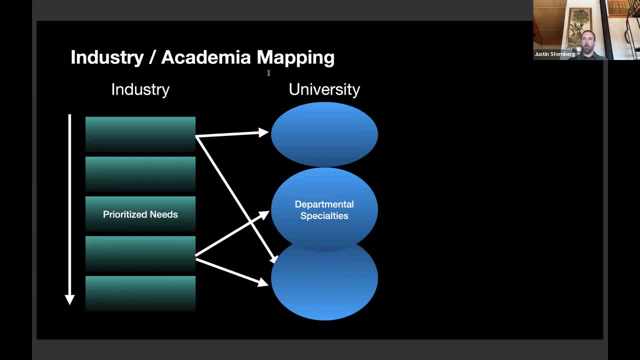 So developing those conversations, getting people comfortable with one another and understanding how to work collaboratively is part of the activities that ABEC is working on. In our gap analysis, we're identifying areas where there's a need for industry expertise that the university doesn't have. I'm going to talk a little bit about that, because 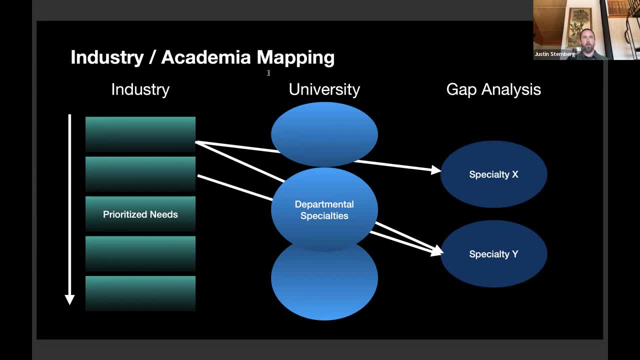 there's a process for developing that. It's easy for us to partner externally with outside of Alaska that have those areas of expertise And in many cases that's beneficial. There's a lot of great partners that we have that are interested in working in Alaska. 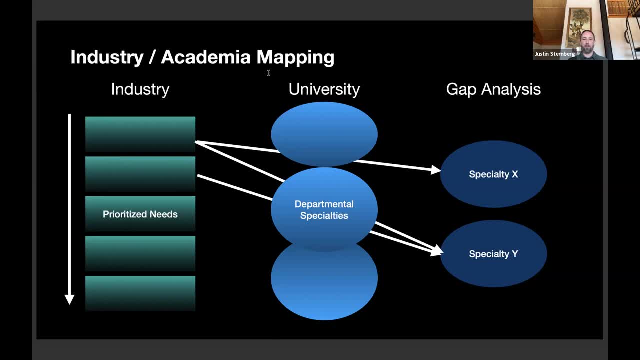 We don't see ourselves really as competing, because Alaska is very unique in the research world And so there's a lot of interest there. However, there's also instances where there's specialties that would be extremely beneficial to develop in-state And looking at ways to create that within the 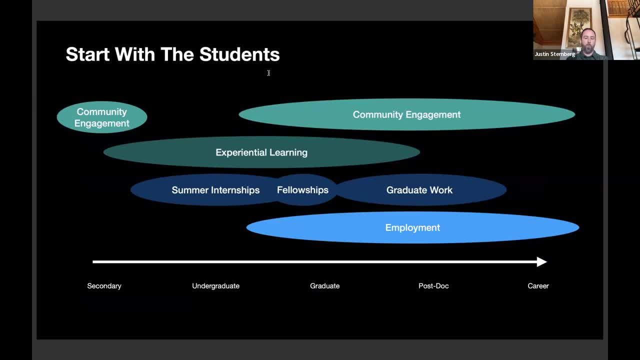 university system is part of what I'm doing. One of the issues there is that going in and talking with the department and researchers- everybody's extremely busy So even if I come in and present on industry needs and the opportunities for work to happen there, most of the researchers are. 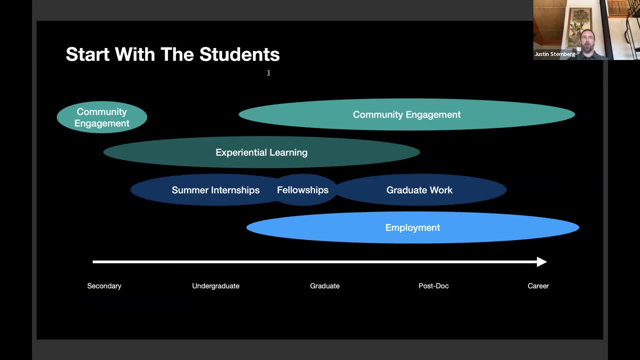 operating at more than 100% capacity, especially with all the research funding that's been made available over the past Three or four years. And so there's a challenge to get people's attention at the staff and faculty level, And the best practice there is to actually start with the students and engaging with the 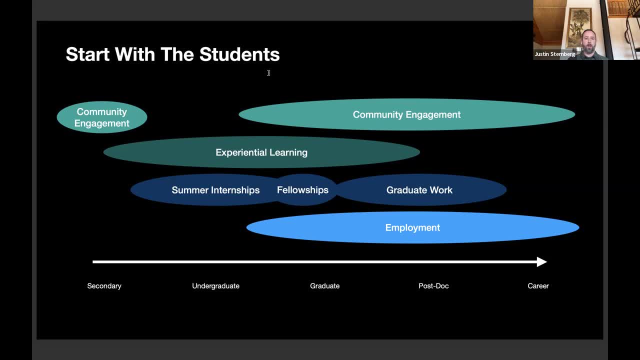 students. That can begin with community engagement, And this can happen as early as middle school or high school. There's a grant that we're working on that's funded by the Office of Naval Research and it's really about building up community innovation hubs in both Cordova and Kotzebue. This is run by 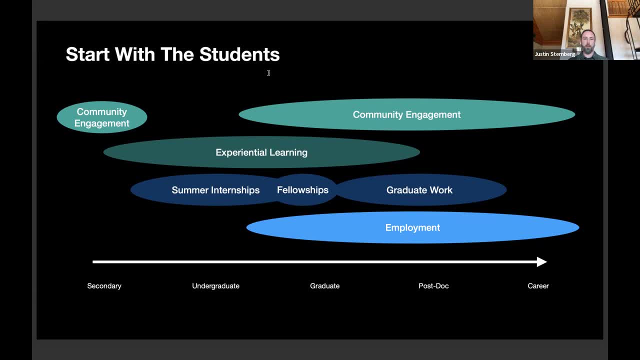 the Alaska Center for Energy and Power. It's primarily focused on renewable energy in those communities And it's really about letting the communities drive the conversation, rather than coming in as outsiders and suggesting what they should do. We do our best to listen to them and 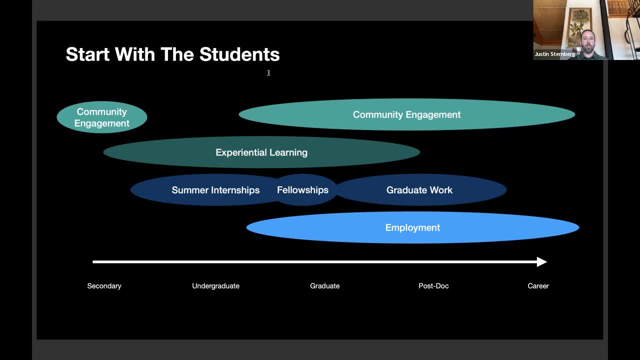 engage with them and provide them research tools that will facilitate them finding solutions for their energy needs. We also recognize that energy isn't the end-all end-all. We also recognize that energy isn't the end-all. We also recognize that energy isn't the end-all. We also recognize that. 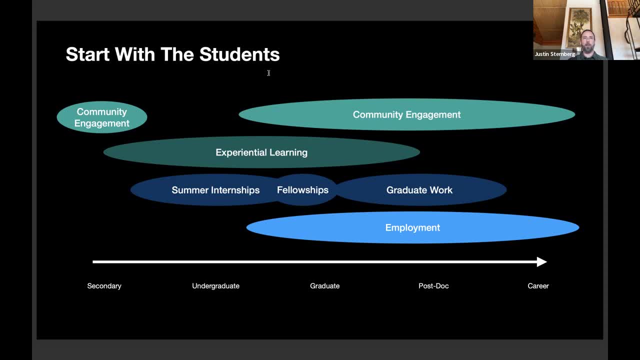 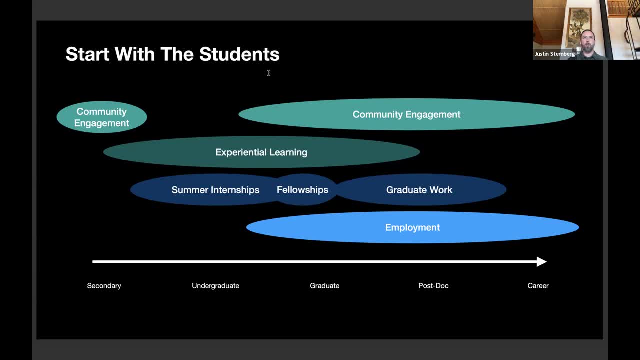 staggering, from some of the lowest costs in the country for electrical power all the way up to some of the highest costs based on whether or not there's renewable resources in these communities that have been developed So that community engagement piece is really key Part of the. 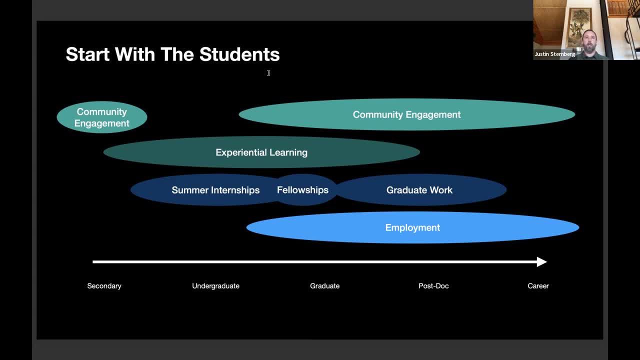 goal in the community innovation hubs is to bring students into the university and simultaneously educating them in areas where the community has identified that there's challenges, and preparing the community to hire the students back after their education so that they can continue to work in their communities and address an ongoing issue in Alaska, which is brain drain. 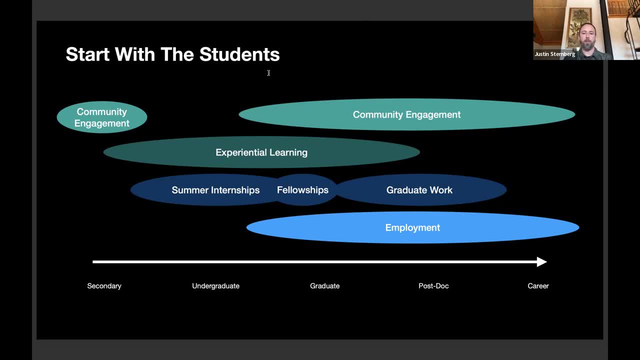 where students that receive a higher degree education have a difficult time coming back and working in their communities. Experiential learning is another key piece here And currently it's happening kind of ad hoc at the class level or the individual professor level. There's some effort to identify ways to expand. 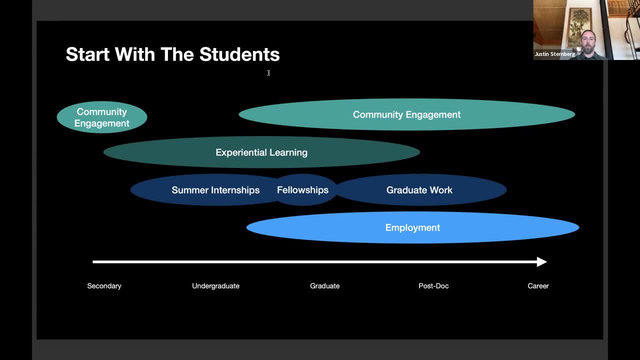 that and to coordinate further with interested parties, industry partners that have projects that they would like to bring into specific classes And a best practice. there is to also maintain some degree of facilitation within the process so that you can ensure that the students are meeting the industry's needs and that the industry is also providing enough time for the 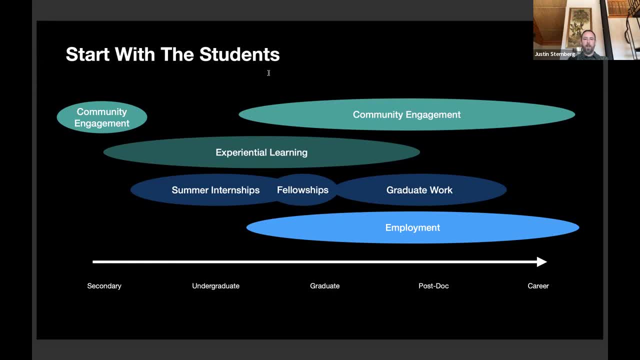 students to get them the information they need. That can evolve into summer internships, as well as fellowships and eventually graduate work partnered with industry partners and then ideally leading to employment with those same partners. There are areas where there's touch points, that we can engage with students in this process. 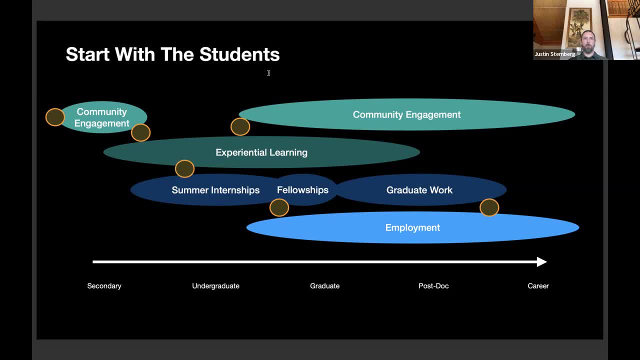 to get them excited about the ocean And for the coastal communities in Alaska. pretty much all the communities in Alaska, including those that are inland, are actually they're also on river systems. So almost every population center in Alaska has some tie to the blue economy and these are areas. 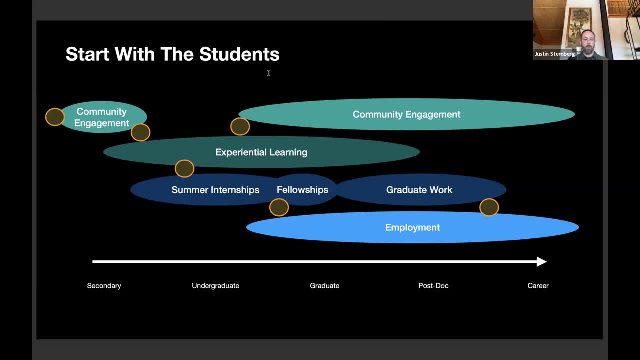 where we have opportunities to engage With the students and bring them into, make them aware of the opportunities of the blue economy and how that relates to them, And we've seen a lot of excitement they're building And so, for instance, with our community innovation hub partners, we're developing. 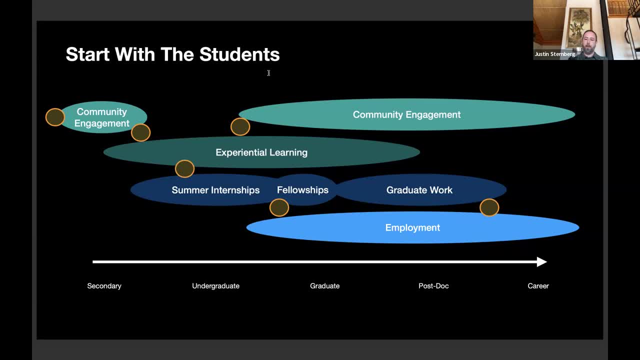 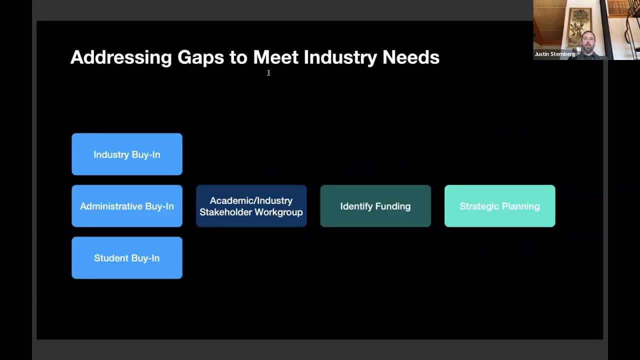 a mariculture curriculum that could be taught at the high school level and engage students while they're in high school, So addressing those gaps to meet industry needs. once we get the, once we have the students on board, it's easier to bring their teachers into the fold, And that in turn engages industry and administration as well. 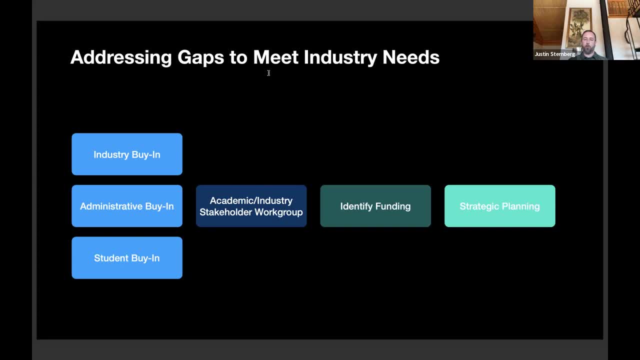 Then setting up an academic industry stakeholder work group would be the next step to talk about ways to develop critical areas within the university, Identifying funding for those areas, which could start as simple as just providing some electives I'll talk about. 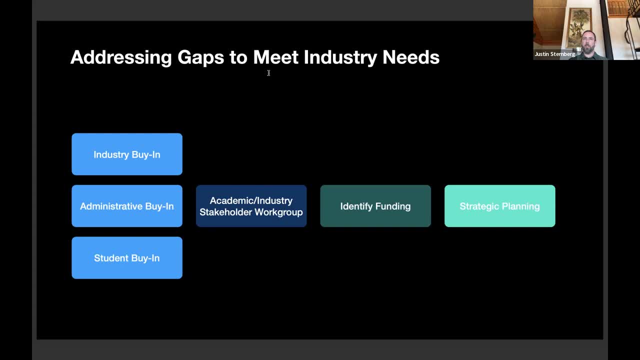 mention ocean engineering in a bit here, but some early discussions about including some electives within mechanical engineering as a starting point for creating that field of expertise at UAF. And then, of course, strategic planning, And sometimes that's very agile, Like when the case of the Alaska Blue Economy Center. we're building the airplane as we're flying. 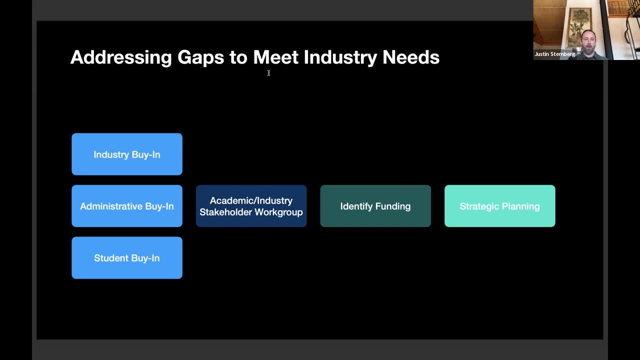 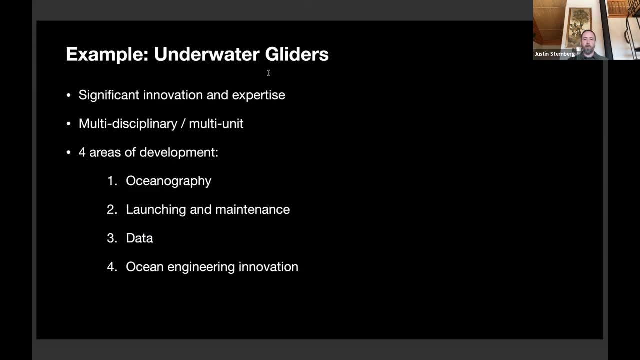 it, so to speak, And so it can happen on the fly, as necessary, to be more responsive. A couple examples here where this is taking place. Underwater gliders is an area that shows tremendous promise for delivering better information from within the ocean. 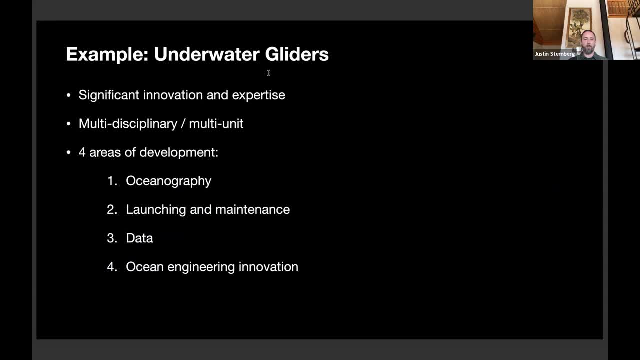 There's significant innovation and expertise at the University of Alaska Fairbanks in these areas that are and it's spread across multiple disciplines and multiple units. In many cases they're sort of collaborating but there's opportunities, I think, for alignment and developing a broader Alaska statewide initiative and going after funding. 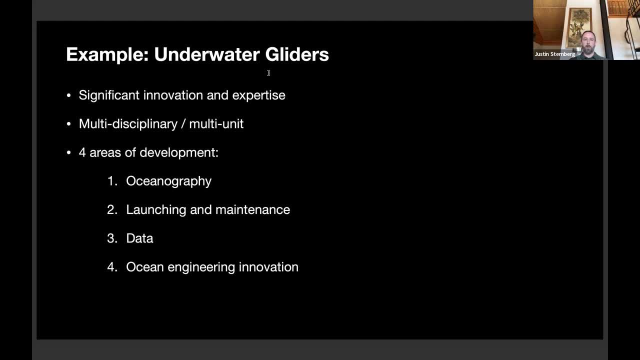 There's four key areas of development. Oceanography is primarily where it's focused right now. There's also the launching and maintenance of the drones and the data platform that I referenced earlier in regards to the increasing amount of large data sets that are becoming available in the future. So those are the two areas that we're looking at, So I'll get to. 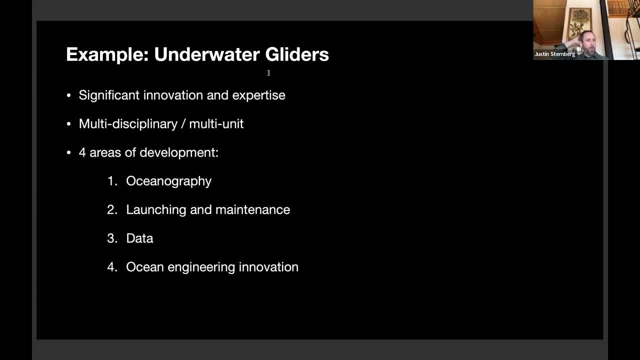 essentially exponential, exponentially growing amounts of data. for instance, one of the glider fleets, the UAF oceans lab within the college of fisheries and ocean sciences- has a single glider that's looking at fisheries issues and working with partners and industry partners to identify opportunities for real-time quota management using the gliders. but they believe that they need. 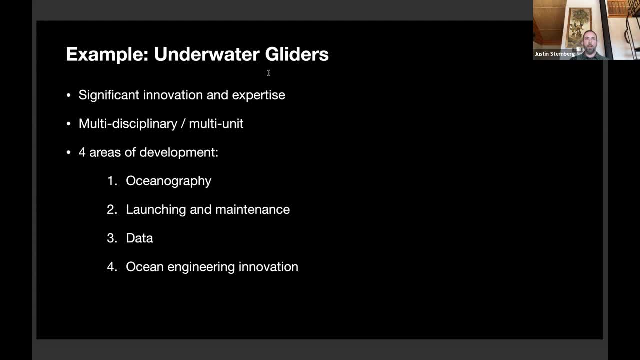 an order of magnitude, more gliders, going from one to at least 10, in order to get a level of data saturation where it would have the predictive qualities that would be necessary for industry's needs. there's also ocean engineering innovation. that happens both on the sensors and 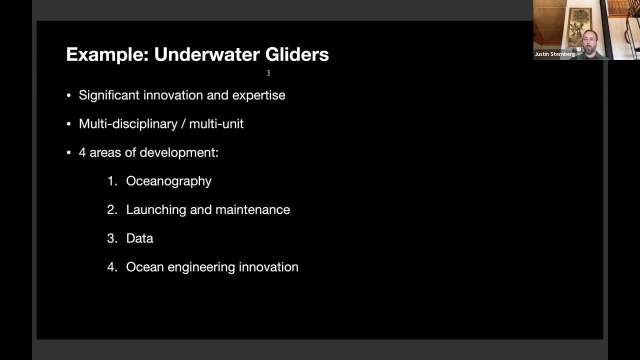 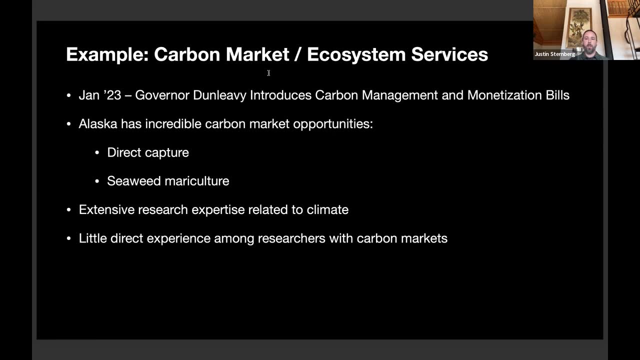 the gliders themselves and, as I mentioned, that's an area that we don't currently have at the university. Another example is the development of Alaska's carbon market and the potential for monetizing ecosystem services, essentially putting the vast, relatively intact ecosystems in Alaska on its 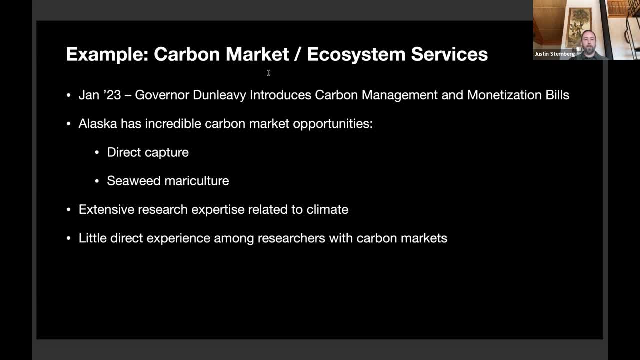 balance sheet this past, this January, Governor Dunleavy introduced the carbon management and monetization bills that would set up a framework for governance of a Alaska-based carbon market and there is incredible opportunities in the direct capture both from our export of energy resources, but he also identified seaweed mariculture as a primary opportunity, given the amounts of carbon. 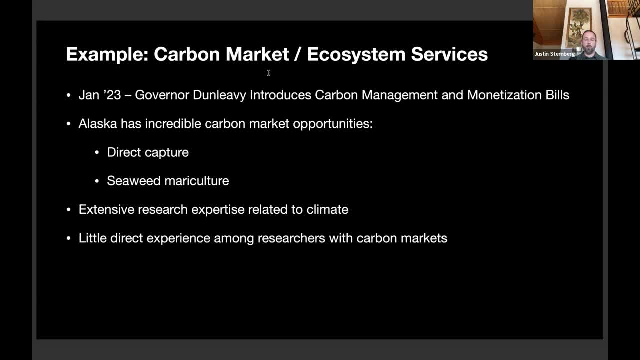 sequestration that are involved when you get to seaweed mariculture at scale. There's extensive research experience expertise related to carbon sequestration. There is extensive research in跟你 to climate in this regard, but we have little direct experience among researchers. 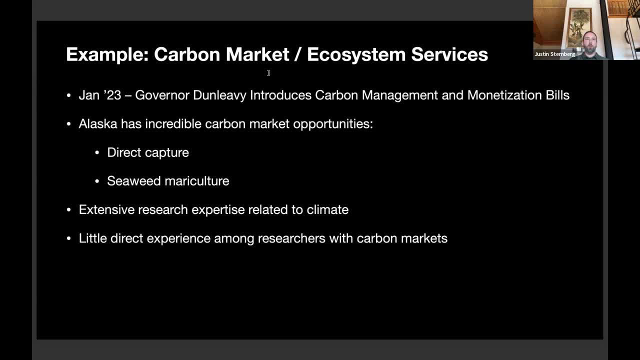 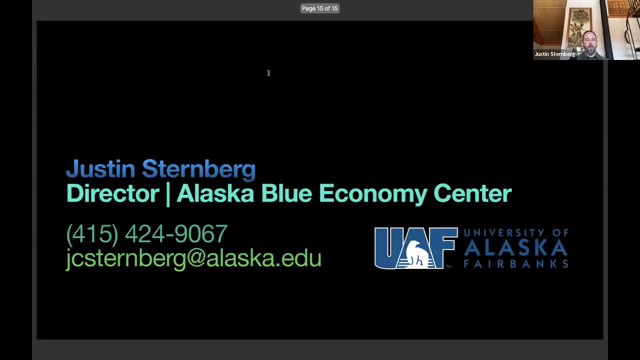 with carbon markets. so in the future you could imagine like a certificate based on like life cycle analysis or monitoring, measurement and verification, two key components for developing carbon expertise. there's my contact info if anybody needs it. thank you- yeah, thank you for just michael and justin for uh taking time off your busy schedules. 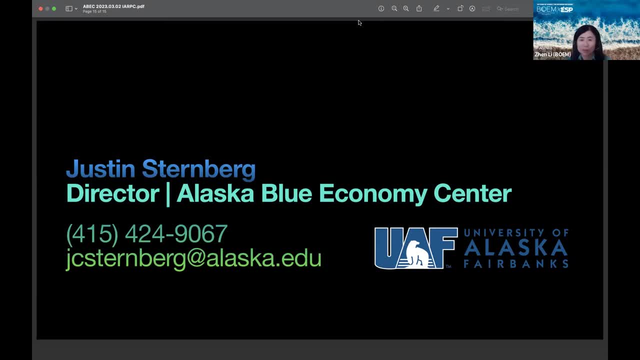 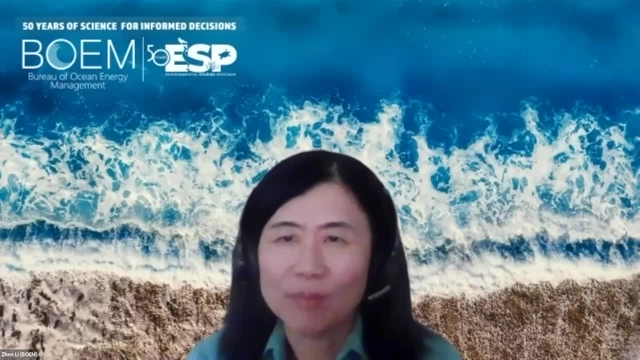 to give us this opportunity to present uh the blue economy and the mariculture of uh sugar cap um in alaska. uh also, um, we'd like to thank for michael, because, um, he actually is calling from tasmania, australia. it's like 5: 00 am in the morning, so let's uh i i thought um, i would like to thank michael and justin for taking time off your busy schedules to give us this opportunity to present the blue economy and the mariculture of sugar cap. um, thank you for justin, for taking time off your busy schedules to give us this opportunity. 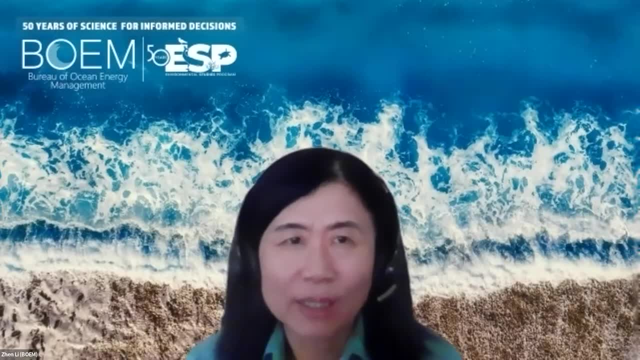 um, i think there's a couple of questions uh to mike. you want to address them, because i see that you have some uh change with um a few people on this uh chat. so you can just, um, you know, i'll give some response here. i i answered them in the chat, if you want. yeah, yeah, okay, yeah, yeah. 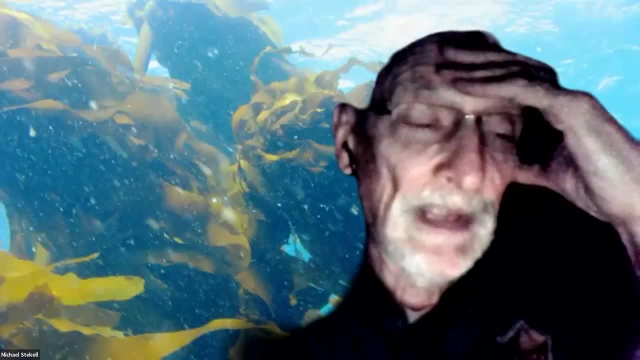 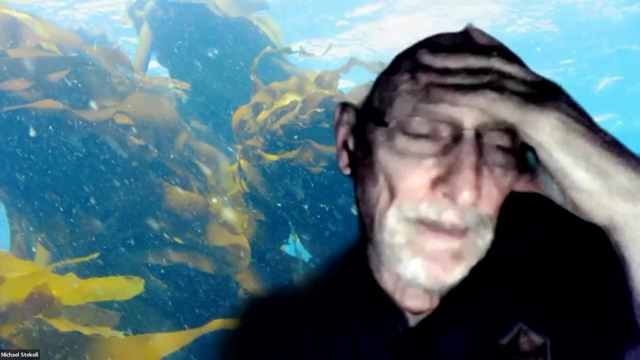 there was an issue about mariculture effect on water chemistry, and it's something that we just. there was an issue about mariculture effect on water chemistry, and it's something that we just don't know enough about it, especially um, if we have very, very large farms, there could be some. affecting me. after all, the seaweeds are are competing with phytoplankton for the nutrients. uh, another issue that mentioned with carbon sequestration: by dropping seaweeds at the bottom of the ocean, seaweeds not only break, take carbon down there, but they're also taking nutrients down. 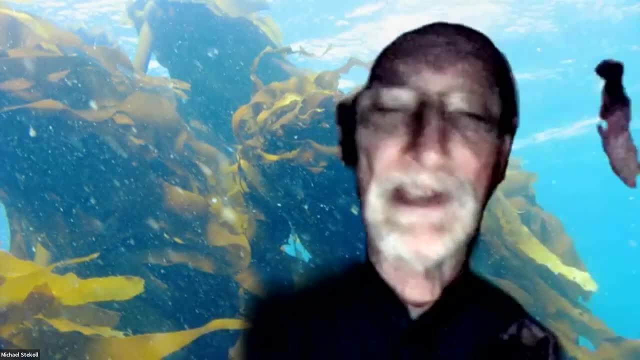 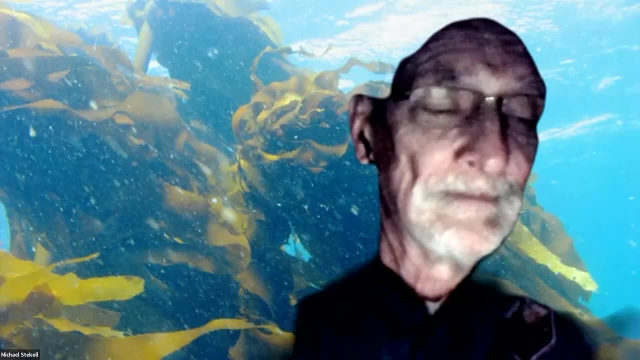 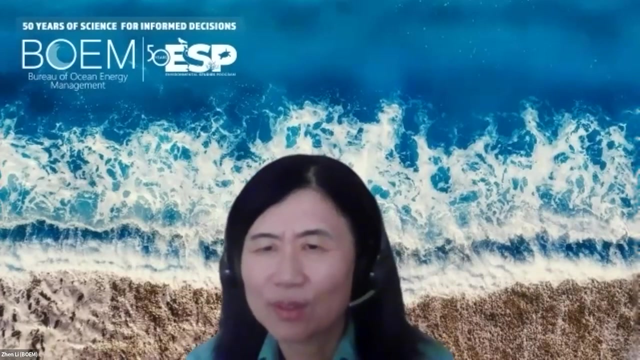 there, so i'm i'm a long way from being convinced that seaweeds is going to be an answer to carbon sequestration. Yeah, let me see if we have any new questions here. Yeah, there's a chat question on Justin. Justin, could you talk more about how you do the industry gap analysis? 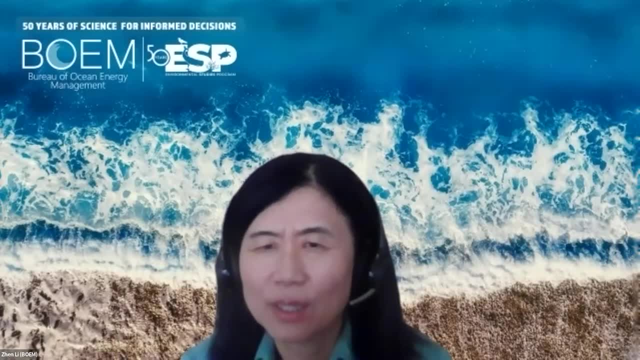 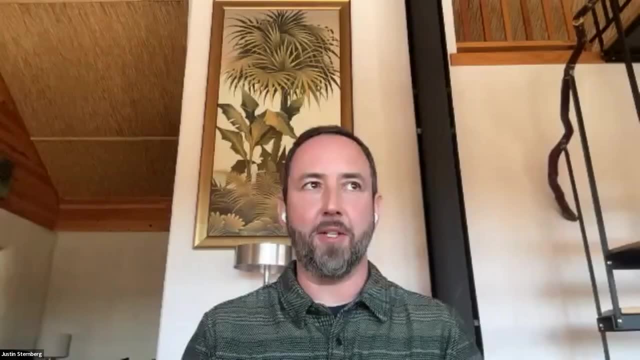 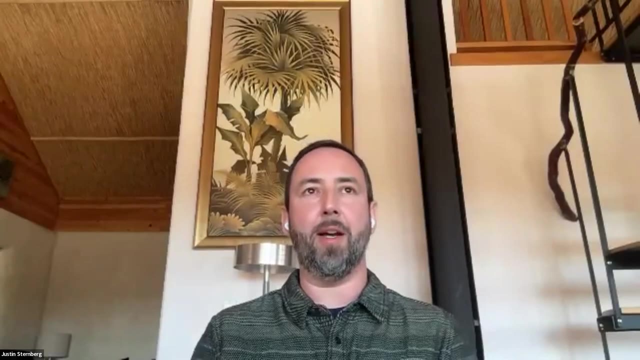 Is that something you do through interviews, more informal connection, building, structured analysis or some other process? Yeah, it's a good question and it's definitely an example of building the airplane as we're flying it. We can point to how it happened at the Alaska Center for Energy and Power. 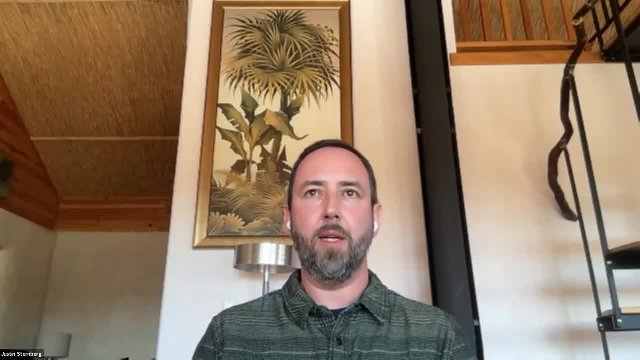 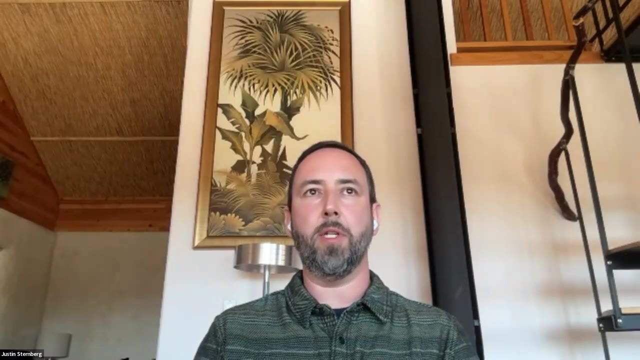 There's some good examples there that are relatively analogous, but it essentially starts working with researchers. We're building a team based on folks that have areas of expertise, For instance, in the mariculture space. we have one researcher named Sherry Umanzor in. 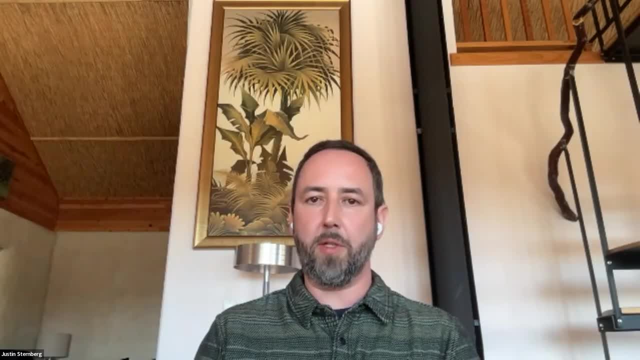 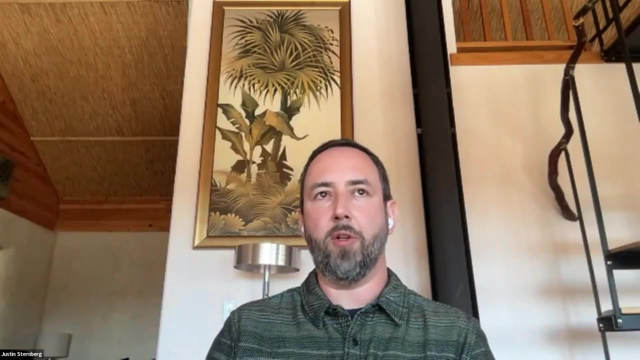 the College of Fisheries and Ocean Sciences, who's focused specifically on mariculture, But then there's also a geneticist at CFOS as well, Jessica Glass. There's some researchers focused on On ocean acidification, And then there's a pathologist in the veterinary school that also is interested in looking. 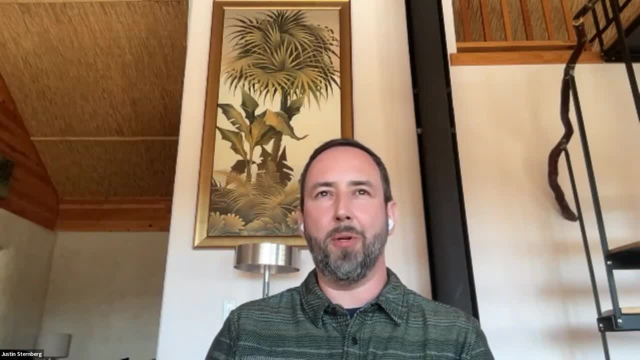 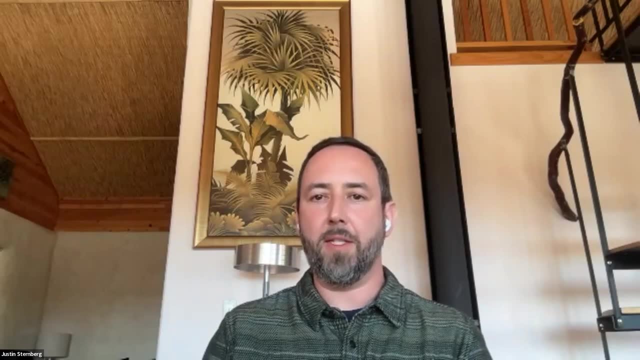 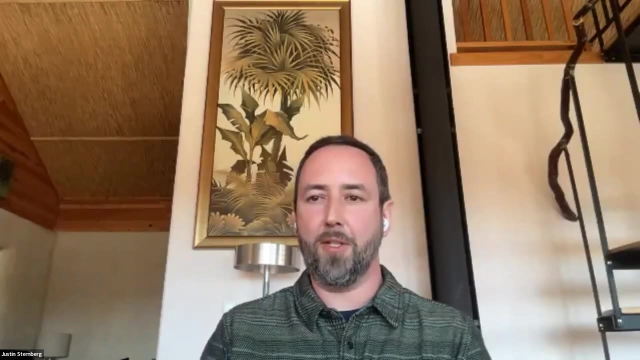 at pathology for seaweeds, And so building out some of those, Building out a team is essentially the first role: People that have skill sets that are relevant and identifying where they are within the university. The UAF isn't a huge university, but every day I learn something new about it. 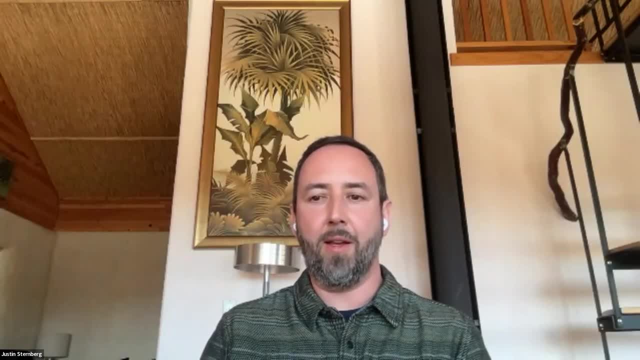 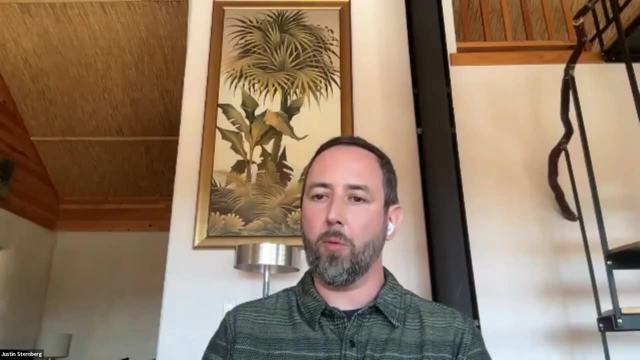 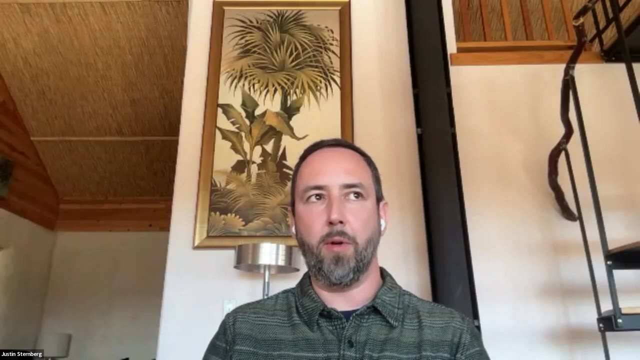 There's an incredible amount of different things happening there, And so it takes some time and it takes networking. I think the next step is to formalize. We've also been doing the same thing. We've been reaching out to industry partners, folks that we've already been working with. 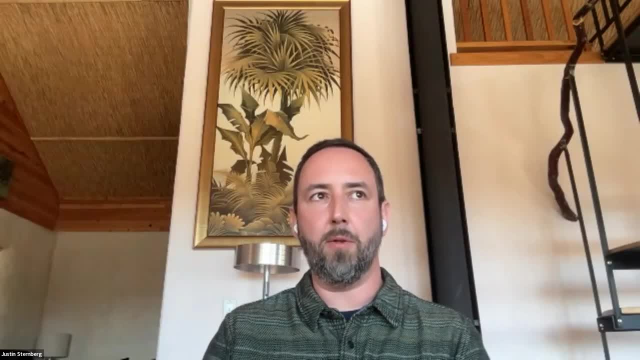 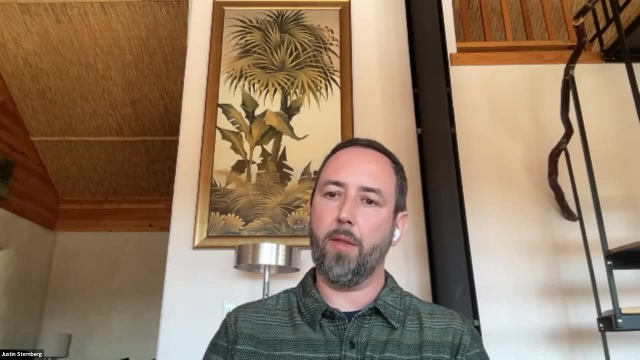 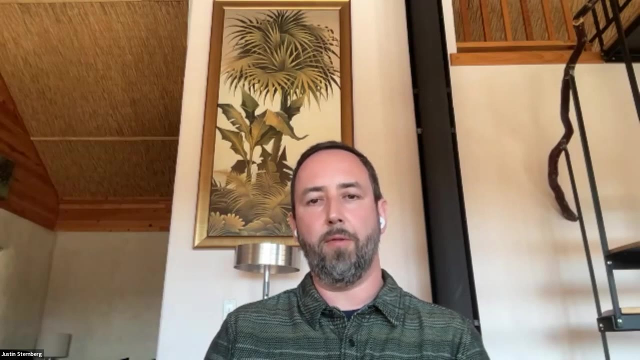 in some cases for many years, But it's pretty broad. So identifying fisheries, Mariculture and seafood processing, I think, are our top three priorities, at least initially, And then bringing together a work group of industry partners and researchers to start to address and look at where the industry's priorities overlap with the university's research. 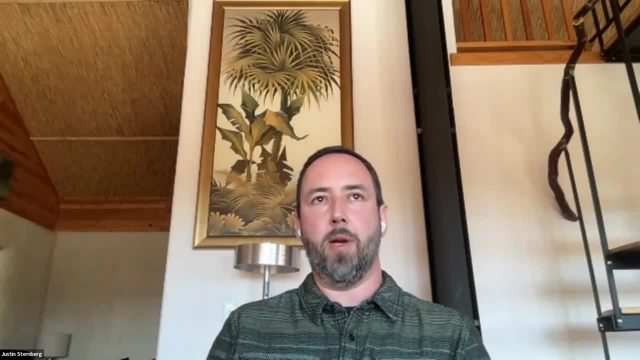 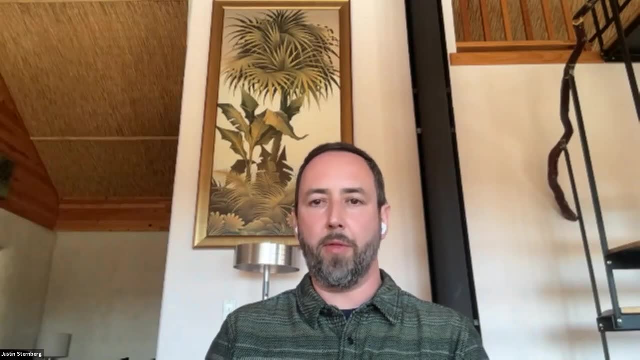 skills And then within that, it's really about conversations within the administration: Talking with- Yeah, I think there's a lot of talk about the ocean engineering example- talking with the Dean of the College of Engineering and Mines to see if he has the bandwidth to take something. 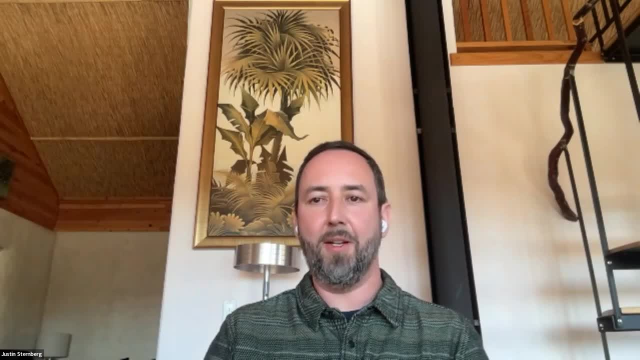 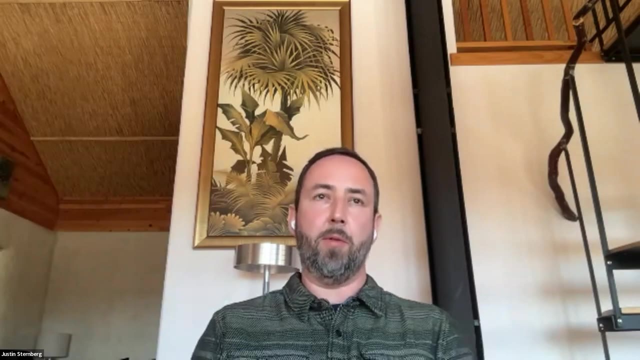 like this on. It turns out he's also bringing on an aerospace engineering program currently, So there's not a lot of bandwidth there, but he also recognizes the opportunity and thinks that there's potential for a stepwise approach. So you can bring in pieces of that. 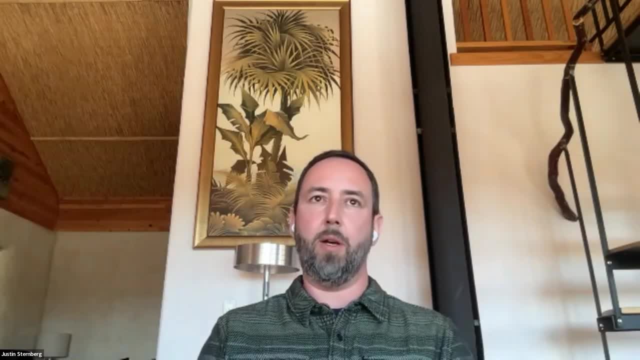 Some of that actually happened when the Alaska Blue Economy Center was formed, So he's bringing in a lot of that, Yeah. So the Alaska Blue Economy Center was first set up, They concurrently created a Blue MBA program with the College of Business and Security. 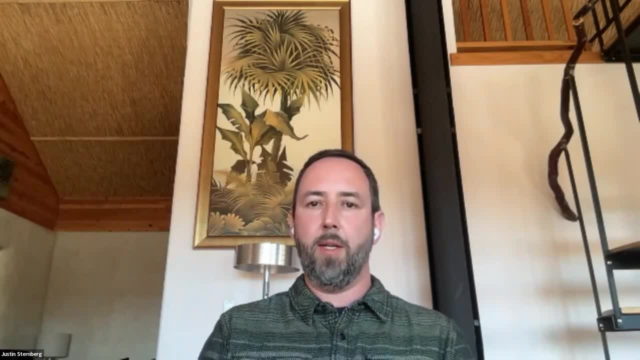 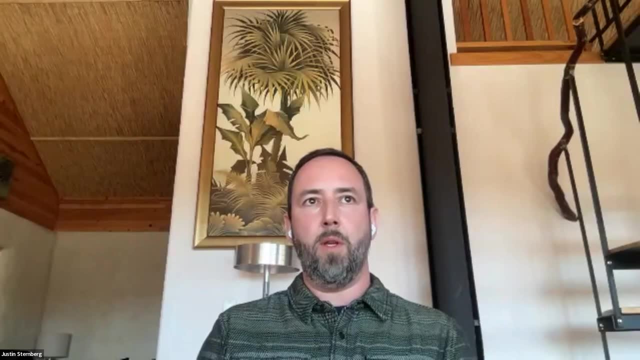 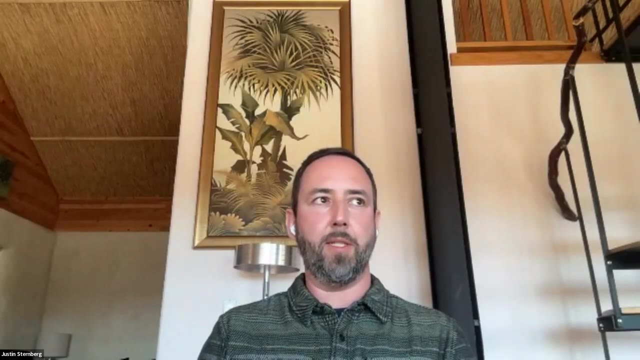 Management, which is our business school, And so that's now getting up and running. It's the only Blue MBA in the world that can be done asynchronously, And I think the only other one that I'm aware of is in Rhode Island, which was also interestingly. 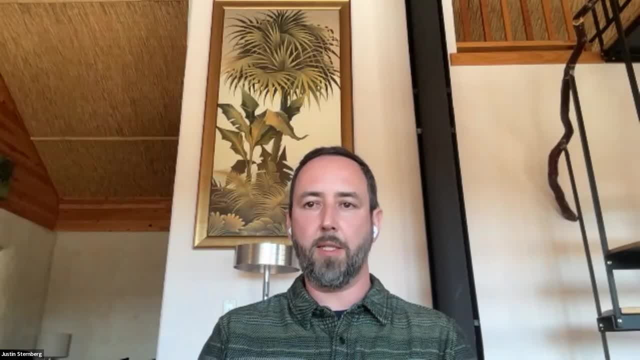 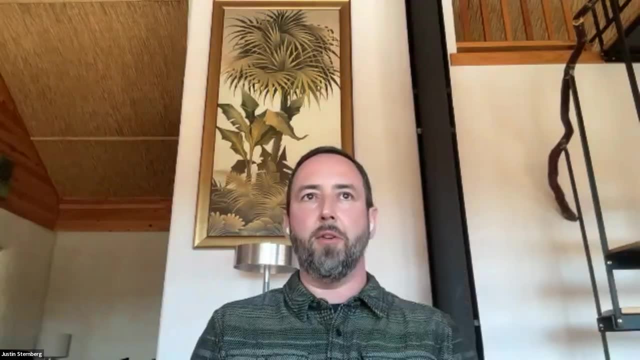 set up by the Dean, Brad Moran of the College of Fisheries and Ocean Sciences. Yeah, Yeah, And so he's now set up two or been involved in the creation of two, And so that kind of it's an interesting approach. 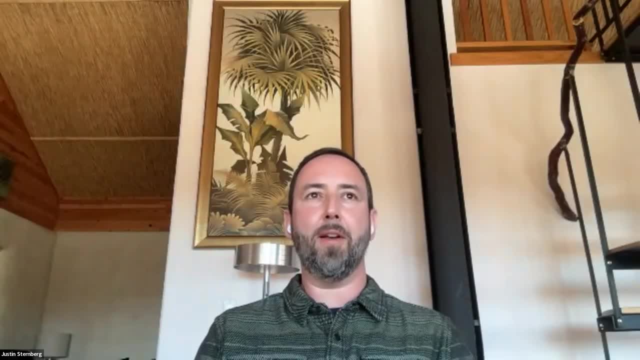 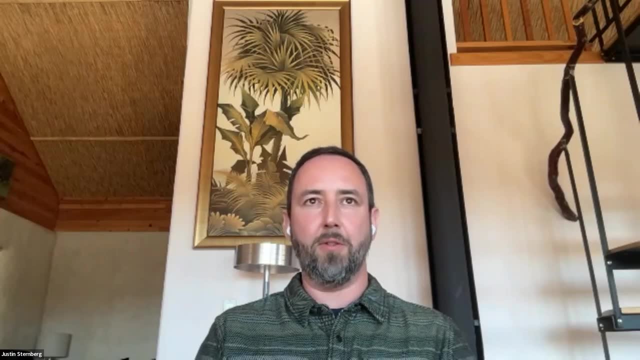 There's- I would almost call it there's- a lot of interest, almost pressure from the state to do more engagement at the community and industry level. There's a lot of needs in the state. Climate change is impacting coastal communities very significantly. 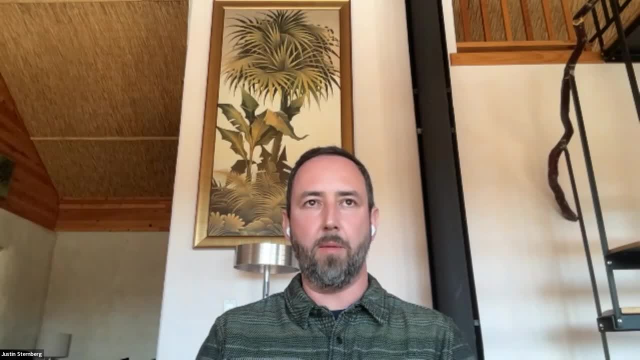 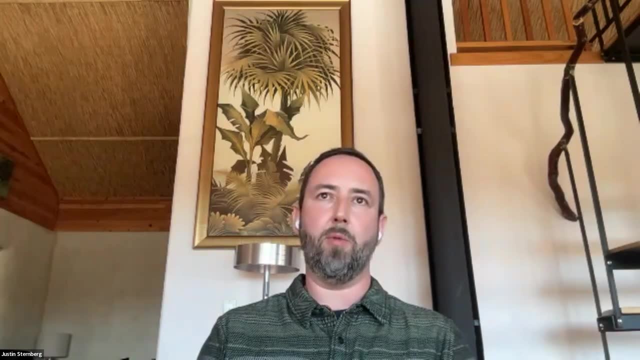 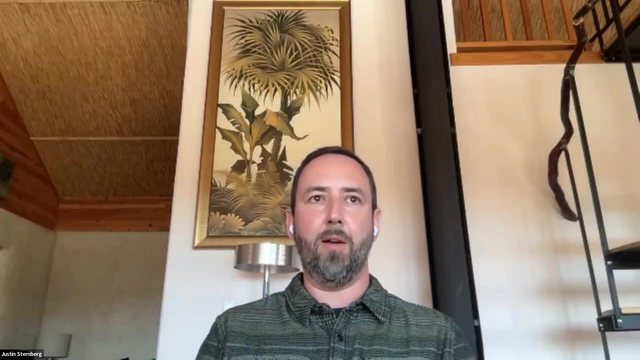 So I think people recognize that. Yeah, I think people recognize the challenge and the opportunities there and there's a lot of willingness to work together And you see that definitely in the mariculture space, where it's very collaborative. There's obviously some competition, but it tends to be more friendly. 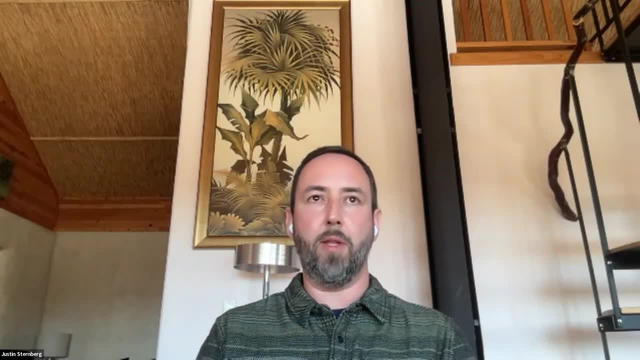 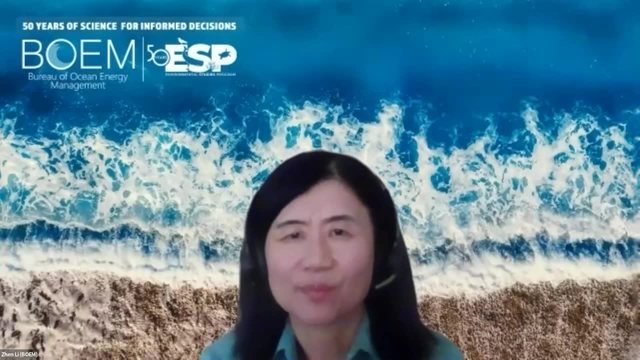 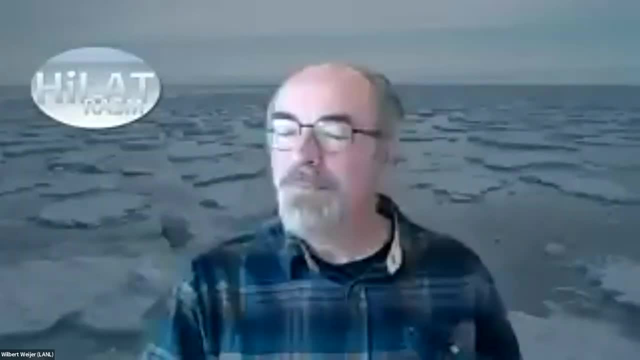 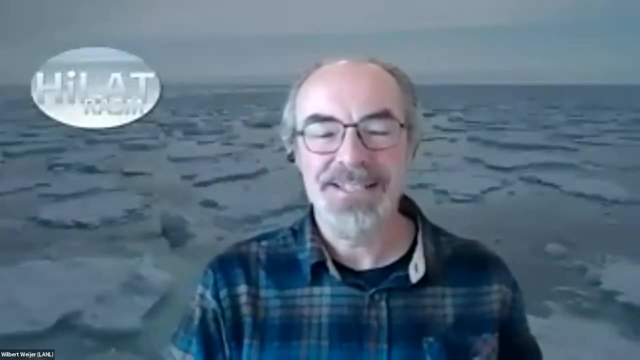 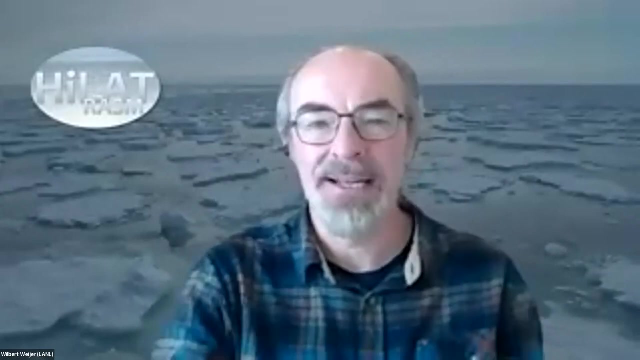 Okay, I saw Wilbert has a with your hand, so please go on. Yeah, So yeah, Thank you. Really great presentations, Justin and Michael. So, Mike, what are your vision? are there the main barriers to really upscaling kelp forestage? 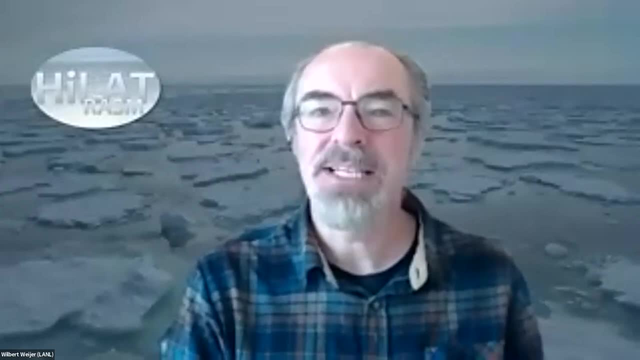 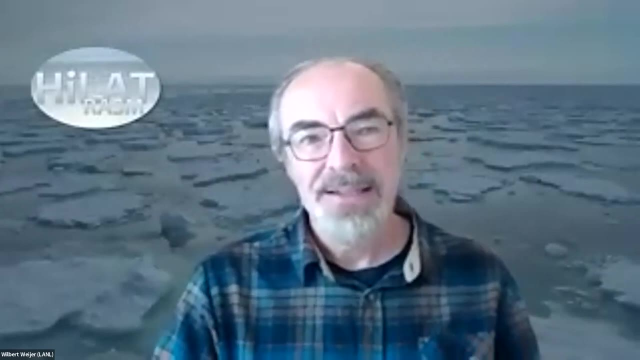 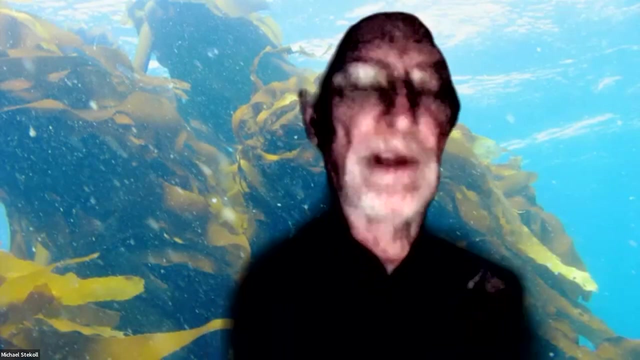 Yeah, farming to really big scale. Is the market a limiting factor there, or is it mostly technology? It would be both, I'm sure, but in order to make larger farms you're going to have to have some markets that lead to larger scale farms. 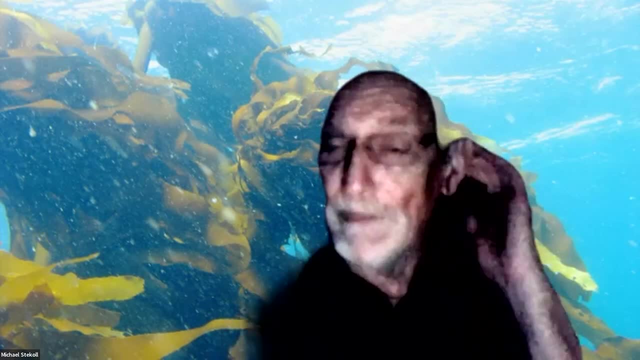 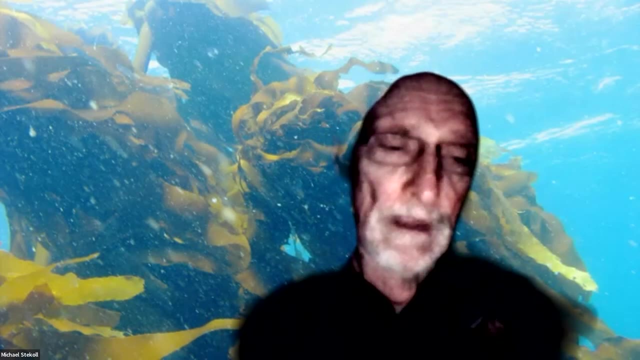 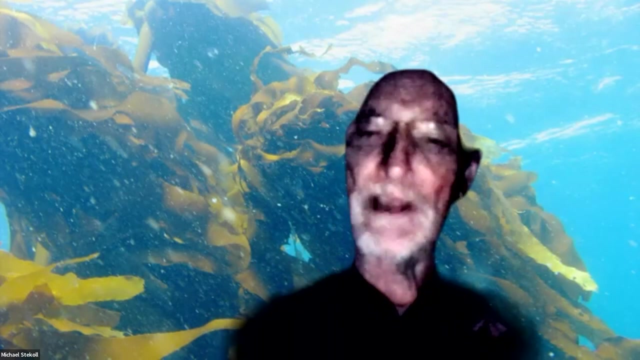 of course, and I don't know what those will be, but bioplastics is one of the things that people are talking about for doing that. and then we haven't actually tried putting structures on the outer coast, and I think that could be a big challenge. 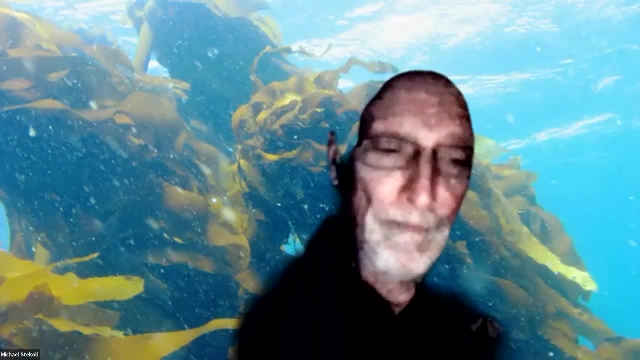 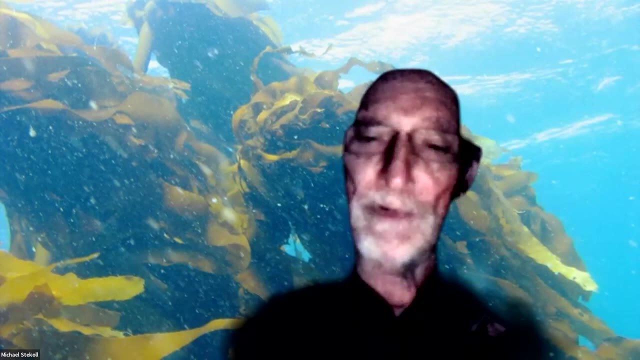 to us and we haven't done that yet. and do we need something like at the scale of oil derricks that are out there, or can we do something that's a lot cheaper and still effective? We don't know yet. People are working on it a little bit. 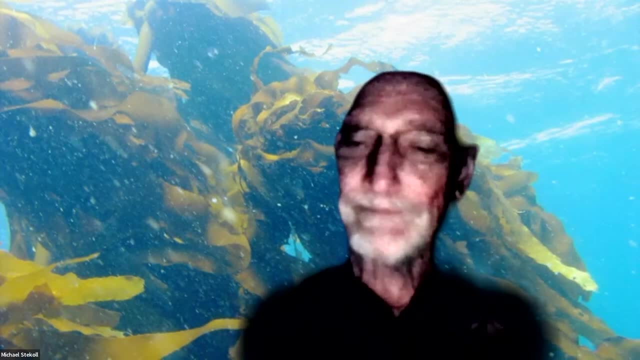 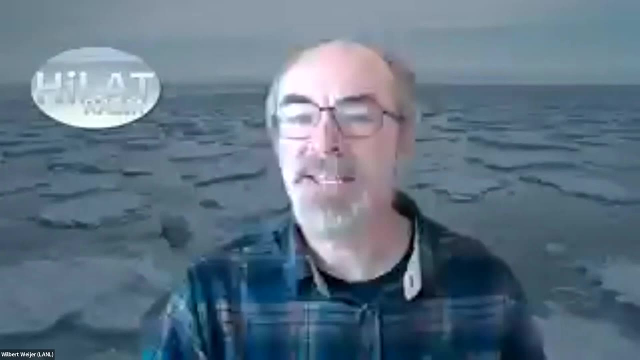 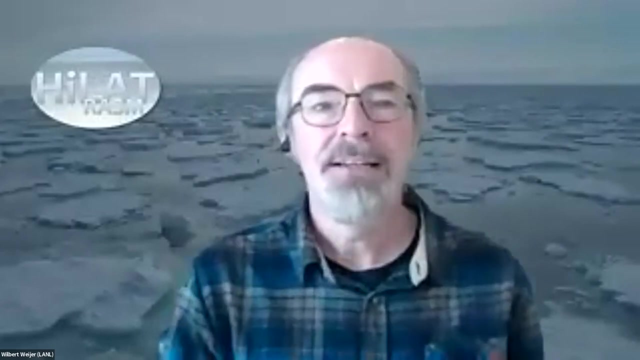 but that's still a long ways to go, I think Great Thanks. Just a follow-up question for Justin. So I mean, if kelp farmers could get carbon credits for this right, then it would help to offset some of the costs, I suppose. and 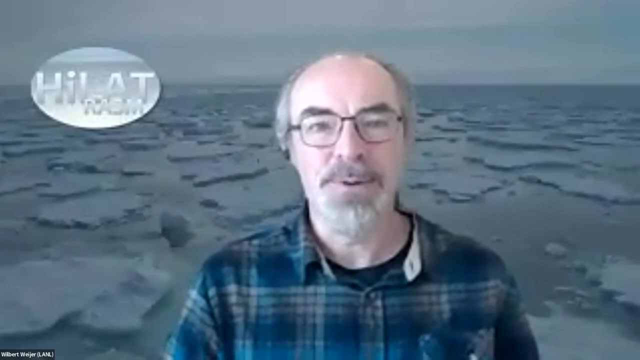 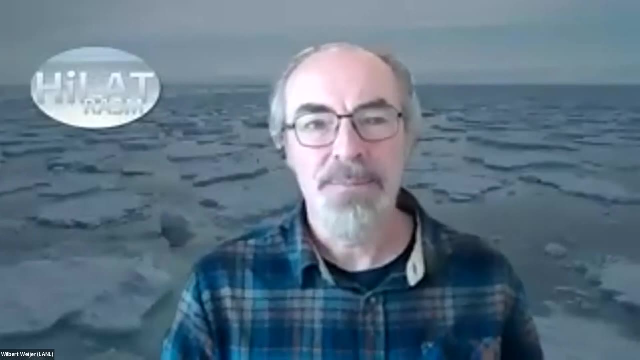 maybe uncertainty in the market. I know that's something that you're thinking about a lot and you mentioned it in your presentation too. I was wondering if you could talk a little bit about that. I mean, is there anything that would be needed? 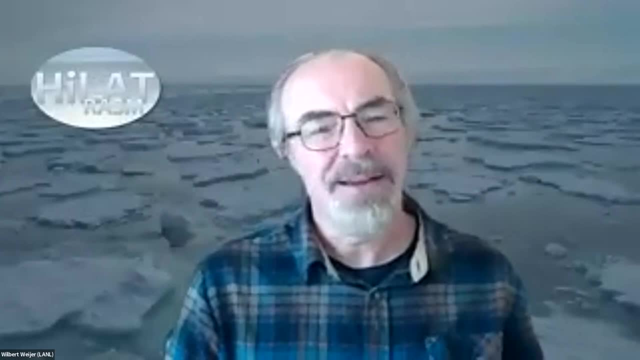 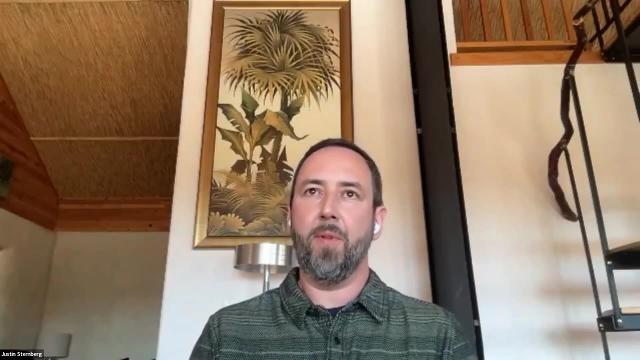 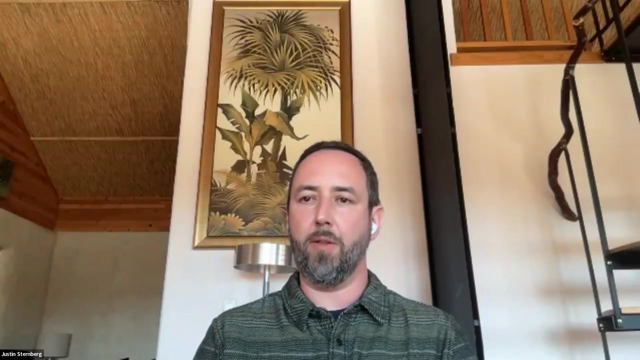 to add kelp farming today to the global carbon market. Yeah, it's well. right now, 99% of the carbon credits are land-based, but in talking with experts in the carbon field, they seem to think that that's actually the inverse of what it should be. that 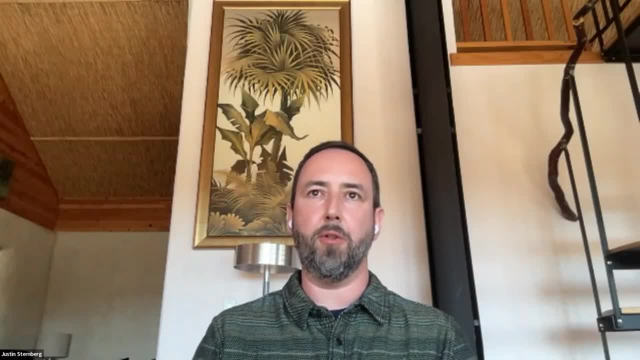 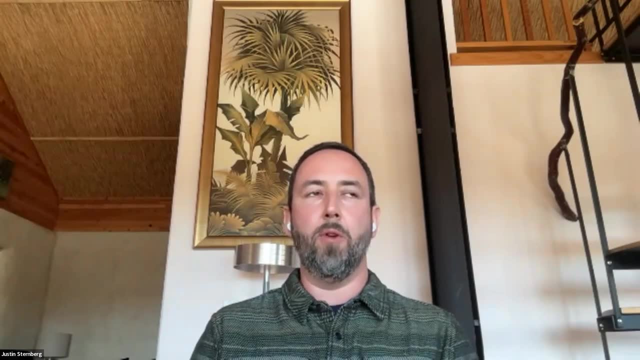 there would be far higher quality carbon credits coming out of the ocean. that would be more impactful to addressing climate change more immediately, And nobody to my knowledge has ever developed a carbon credit based on seaweed, So understanding that what that looks like would. 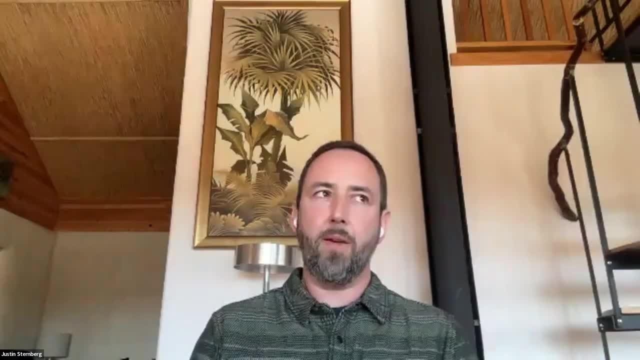 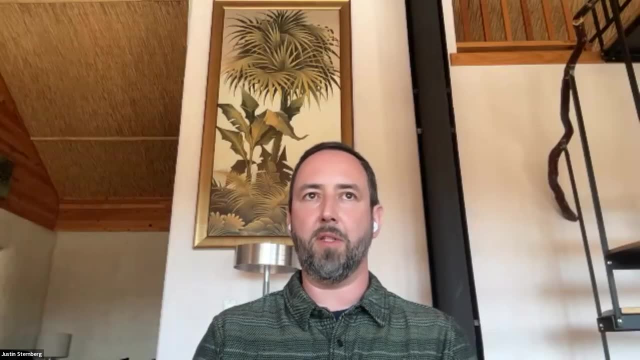 be a good first step And I think- I don't know- that it would ever be a primary source of revenue. but it could certainly help on the margins where you may have. some farmers may have seaweed that's left over that they don't have a buyer for. 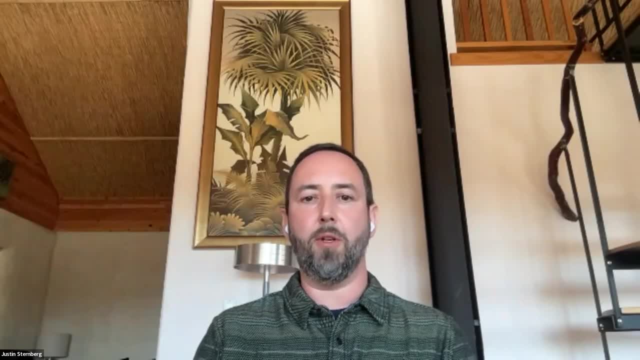 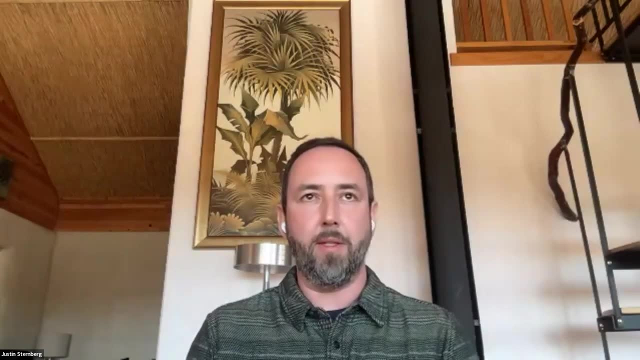 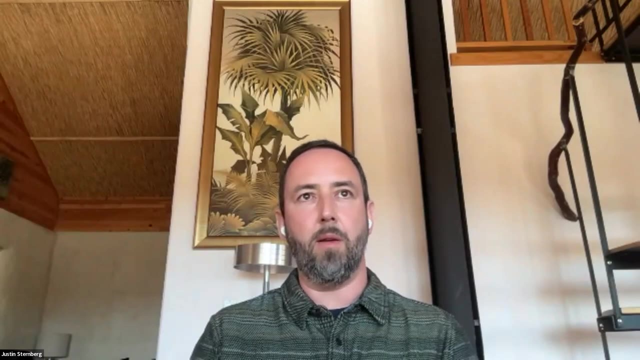 or there may be parts of the kelp that don't have a buyer for. They don't go into the processing that they could use for carbon credits And one of the things that one of the markets for seaweeds would be as animal feed. 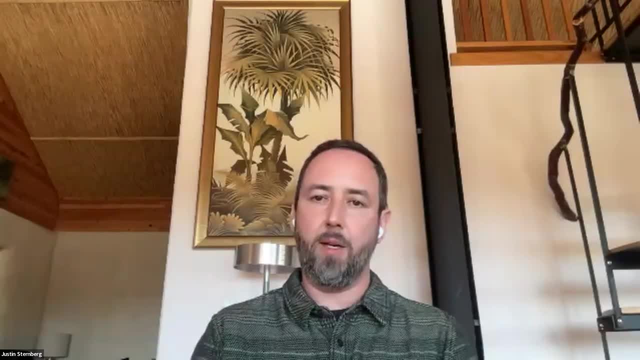 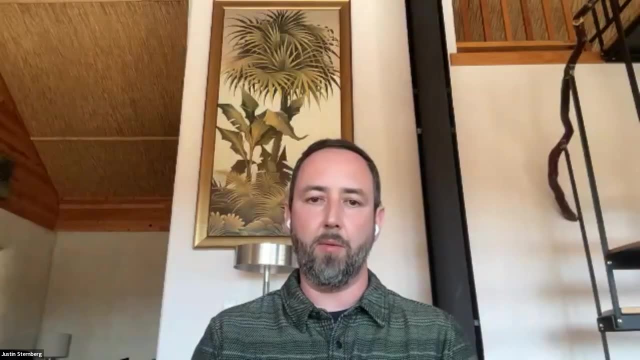 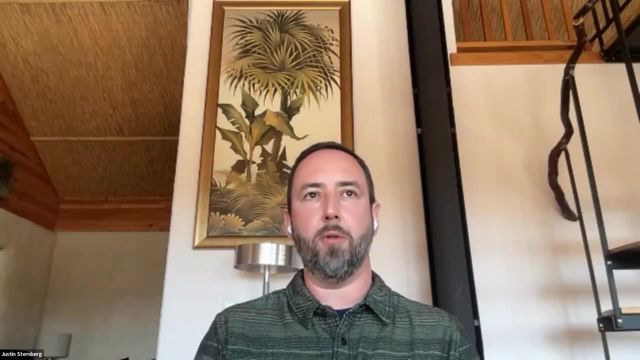 And so it looks very promising from a methane reduction perspective, with some studies showing between 20 and 80% reduction in methane from the animals that are fed a diet that includes seaweed, and also a corresponding reduction in the amount of food that they need to eat. 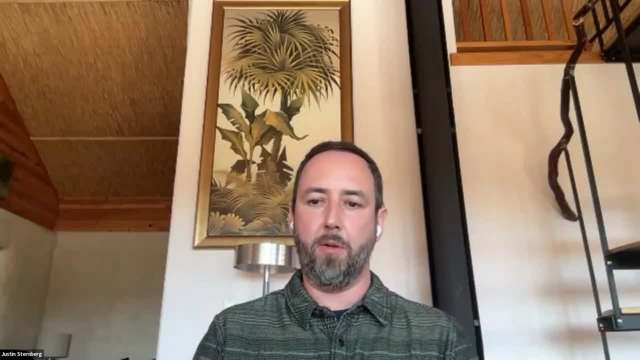 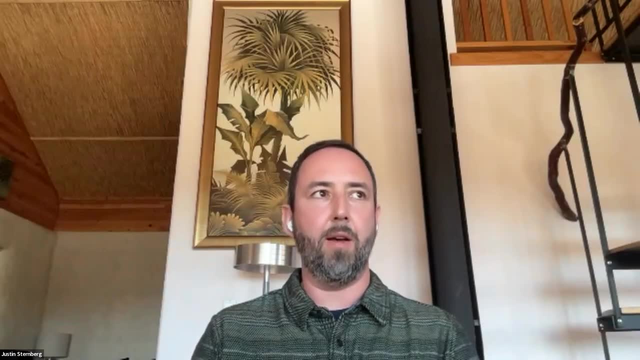 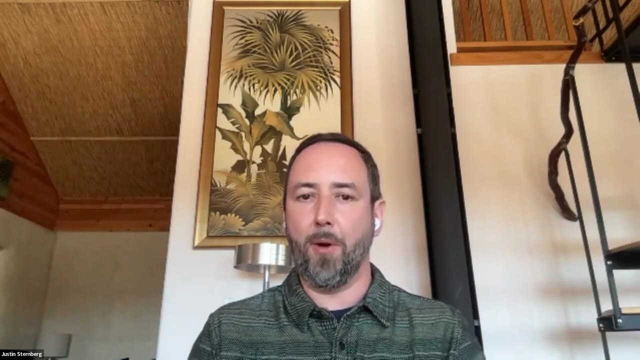 because they're getting better nutrients of about 10%. So that may, with the relationship between carbon and methane being what it is, many times more credit for methane. due to its impact, it may be a better market to go after methane equivalent carbon credits. 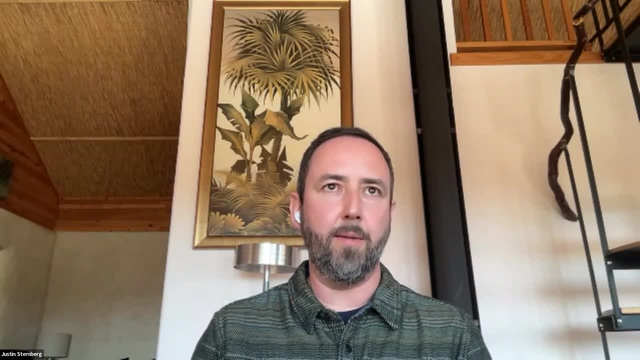 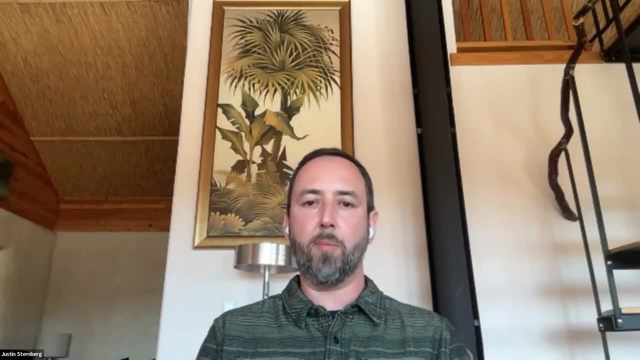 So yeah, it's a pretty big risk factor. It's a little bit more of a risk factor than to think about sinking the seaweeds, At least initially. I know in Canada it's like methane emission from animals is about from farm animals. 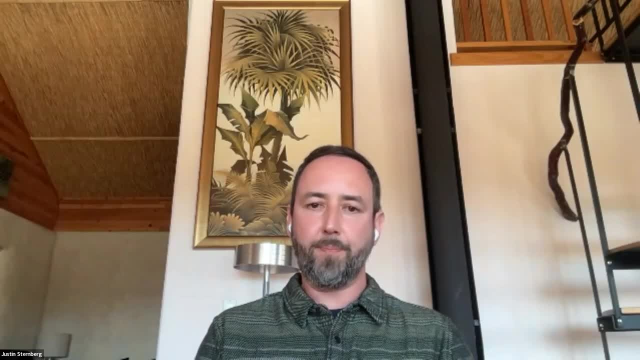 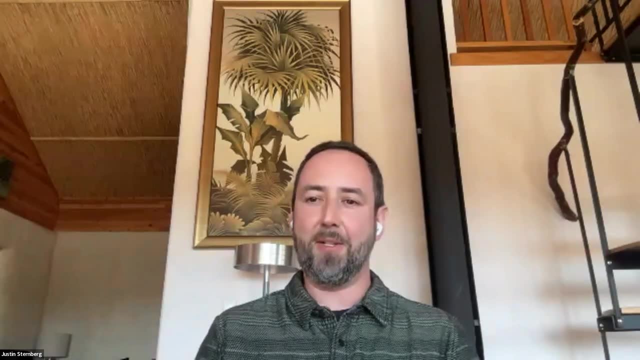 It's about 25% of their total greenhouse gas emission, So it's pretty significant And 80% seems really high. but if you figure these studies depending on the species, it's somewhere in there. It's still fairly significant amount of methane that could be reduced quickly.